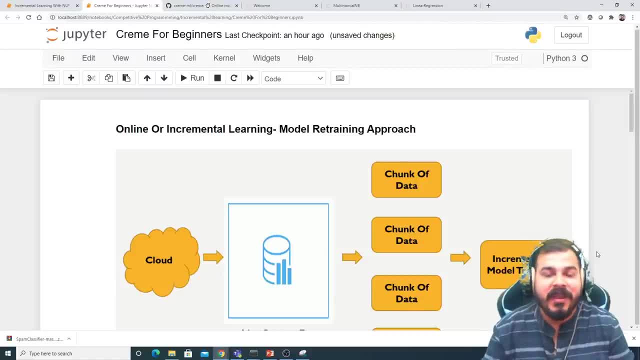 Hello, all my name is Krishnayak and welcome to my YouTube channel. So, guys, from many days, everybody is talking about model retraining approaches. You were requesting me to upload videos on that- how we can understand that, and there is a concept which is called as model. 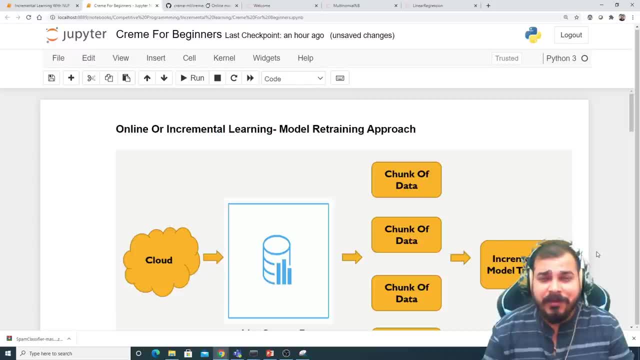 drifting, which I have actually told you. So I am basically going to start a playlist on model retraining approaches. also, guys, There is just not one approach, there are many approaches. One of the approach, which I think that it is better that you all know it, that I'll be teaching. 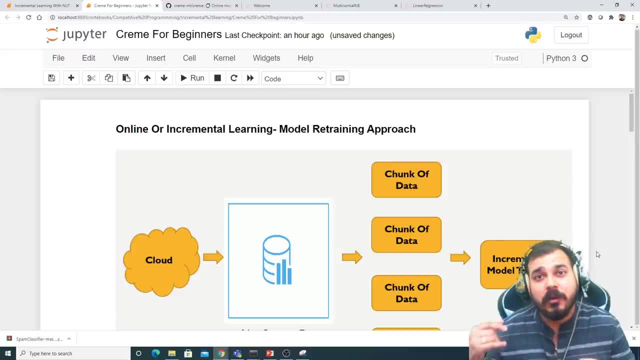 you in this and apart from that, any approaches- and most of the approaches are also been done in- directly into the servers right over there. They have different, different kind of techniques in Azure or in AWS, So I'll be covering that part also in the upcoming videos, but in these videos 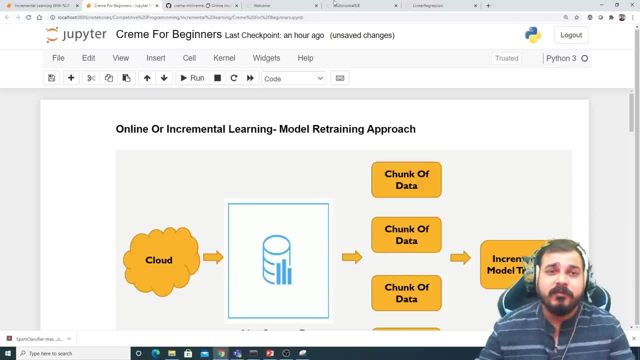 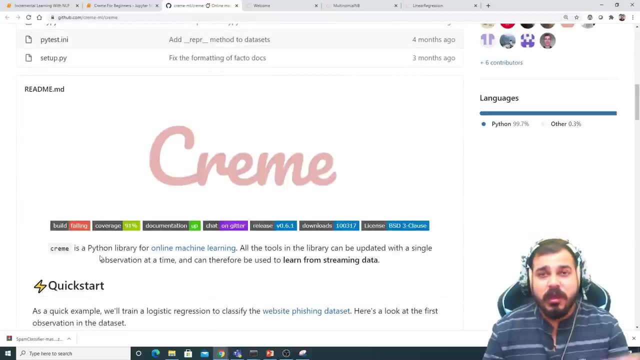 I'm going to introduce to you a very special library which is called as CREME. So this particular library, CREME- it's pretty amazing with respect to incremental model training. So you can see that CREME is a Python library for online machine learning. 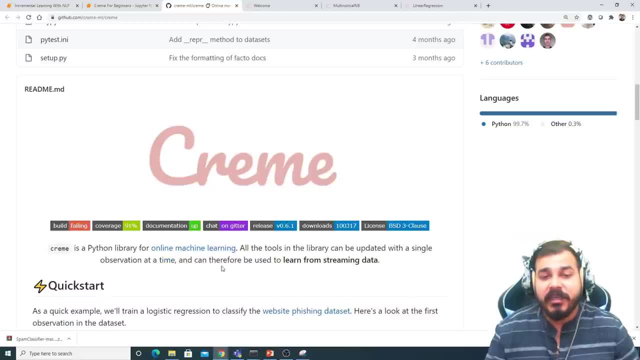 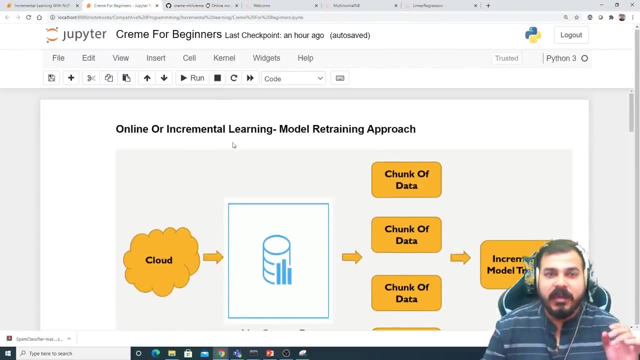 All tools in the library can be updated with a single observation at a time and therefore be used to learn for streaming data. Now, what does this basically mean? Now, guys always understand that, suppose, and what you have learned till now is that you will basically be creating some kind 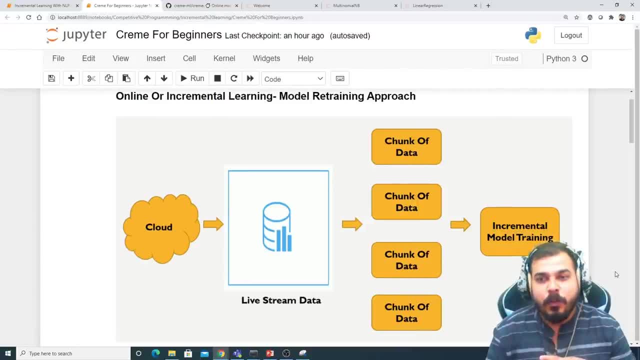 of models. You will be creating some kind of models itself, and when you are creating the model, you are basically using SKLearn. You'll be having some amount of data set and then you will be training it offline, right, and then the model you'll be doing some kind of training, So you'll 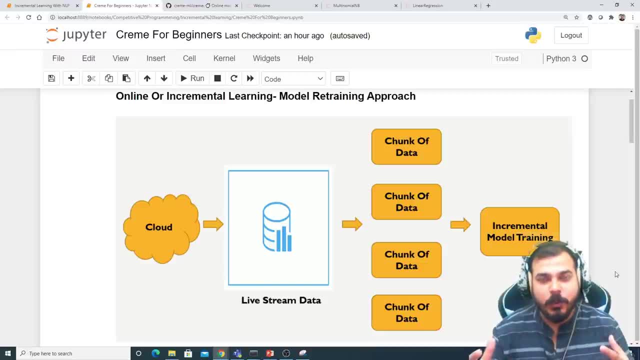 be doing all the lifecycle of the data science project into it and finally you'll be getting some better accuracy and then, when you are ready with that, you'll be doing the deployment, But usually in scenarios, in in various scenarios in various data science project. you know you will. 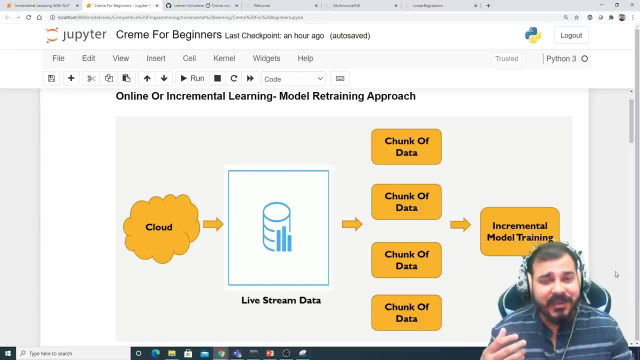 be continuously receiving live data. Okay, every second, some amount of data will be definitely coming, and when those kind of data are coming, you also want your model to get continued, to get trained continuously with respect to the new data And guys, if I talk about bigger companies like 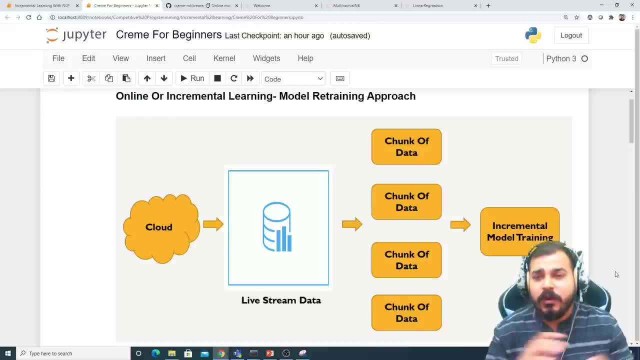 Netflix, like Amazon, they just don't create one model. There will be hundred different models. Okay, and whenever I talk about model retraining approach, this is one approach wherein, whenever we get a new live data, we continuously take it and continuously train it. And yes, with respect, 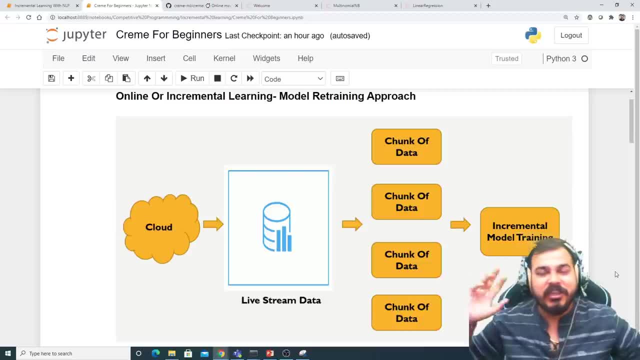 to that again, since there are many models, as such, each and every training data will be pushed into different models and then how that specific training will actually happen. Now let me take some approaches over here and again. there are various approaches. again I'm saying you guys this: 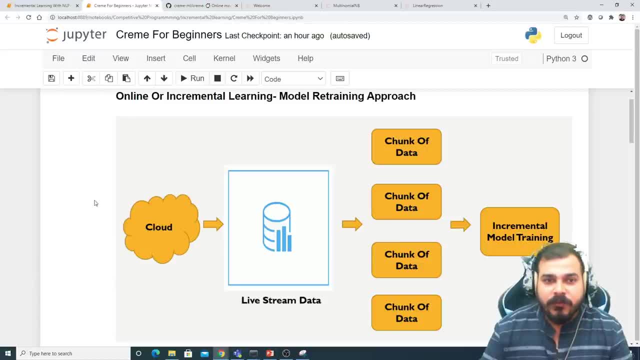 is only the not the single approach. Let me take an example. Suppose from the live stream data. what we do is that from the cloud right we take the live stream data and from this live stream data what we do, we store that efficiently in the big data right and again for storing it over here we. 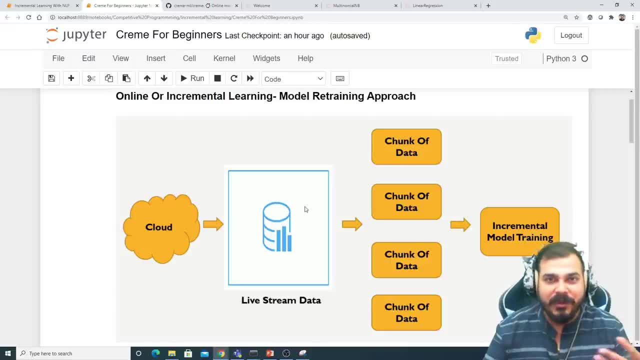 may be using Spark, we may be using different kind of techniques over here For pre-processing and all once that particular big data is, once that data is stored in some kind of databases efficiently, then what we do is that we take those chunk of data and then what we do we 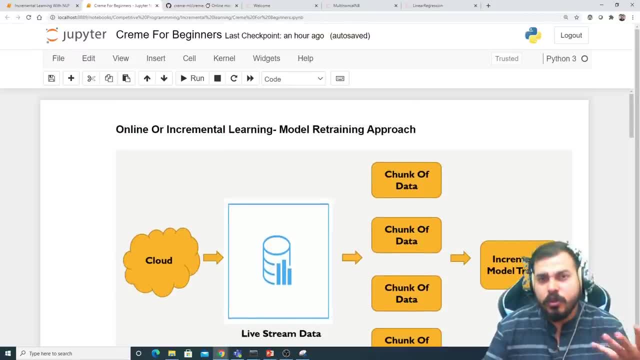 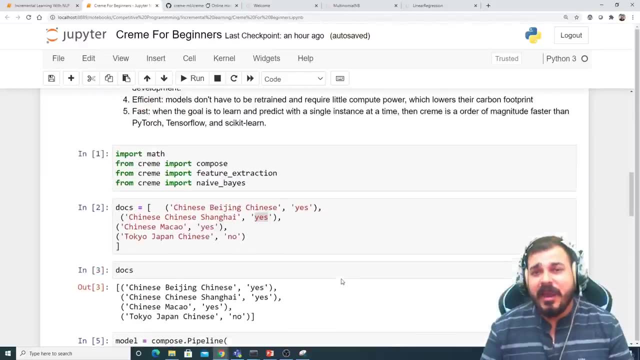 do incremental training, incremental model training? I'll show you that. how does this incremental model training happens in the code itself, and this is what is the whole code that I've actually written, where I'll be explaining about it. I've taken two projects with respect to NLP and, yes, in the future. 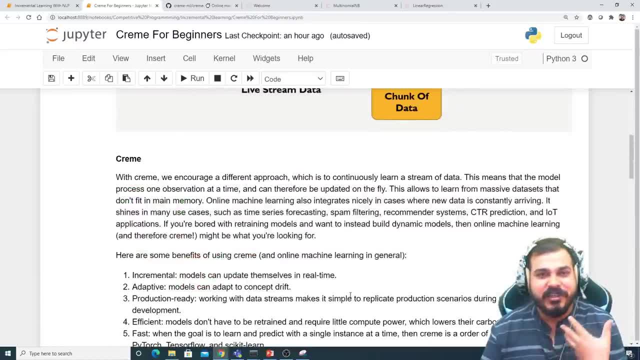 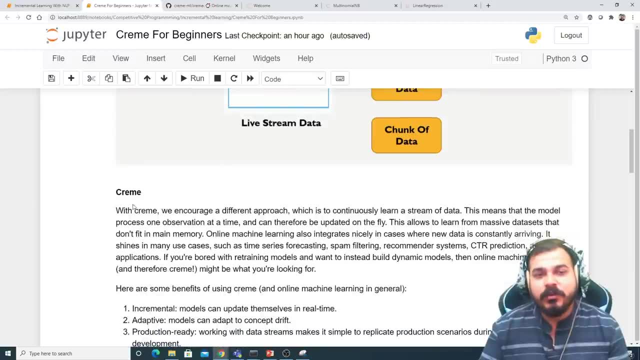 I'll also be taking some of projects with respect to logistic regression, different kind of algorithms like name bias, like k-means, clustering and many more things. So, again, as I said, that we will be using this CREME library again, if you don't know about CREME guys, it is a python library for online machine learning, which is also called as. 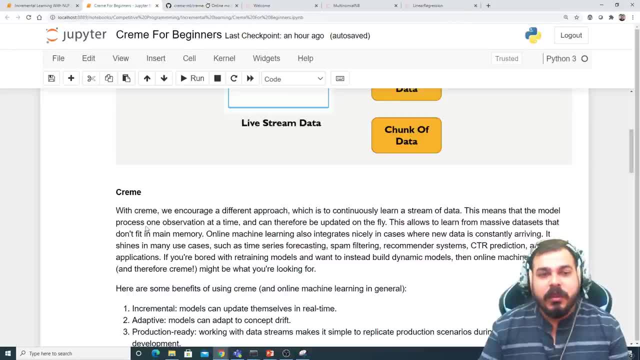 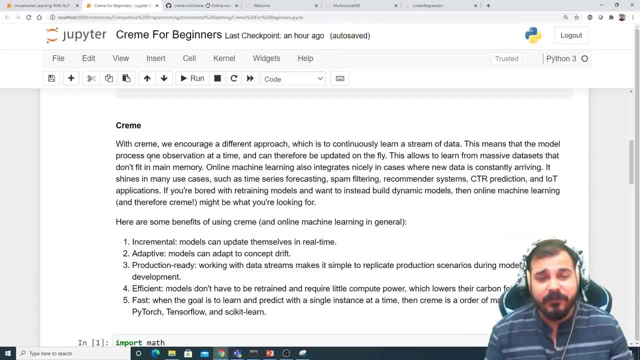 incremental machine learning. There are some advantages with respect to CREME. so we can- we can say that I'll just read this text. guys, please make sure that you watch this video till the end. it is very, very important for every one of you. With CREME, we encourage a different approach, which 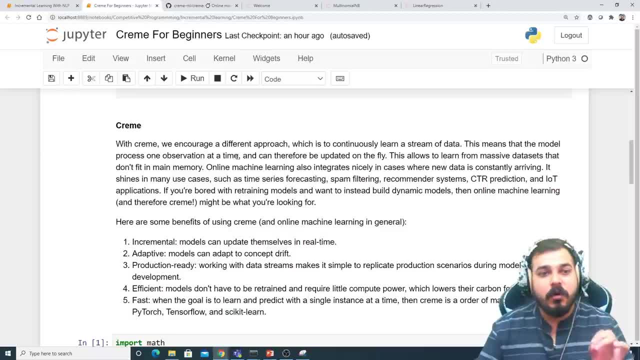 is continuously to learn a stream of data. This means that a model process one observation at a time and can therefore be updated on the fly. This allows to learn from massive data set that don't fit in the memory. so this is also one of the advantages. We cannot just take continuously the whole. suppose if you have millions of data at 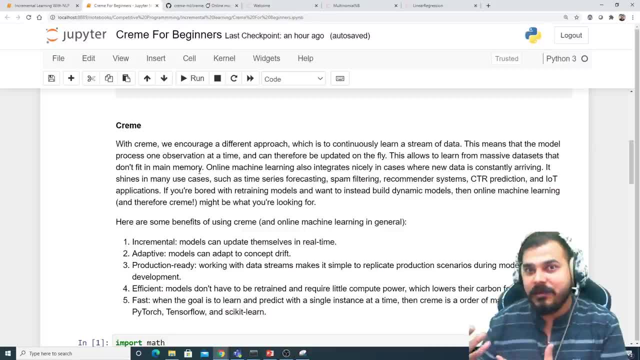 a time right. we just cannot suppose. and in the, in the cloud side also, suppose in the server side or in your local machine. suppose you know that many of you know that you have 16 GB of RAM and suppose you have millions of records and probably you will not be able to fit that millions of records into. 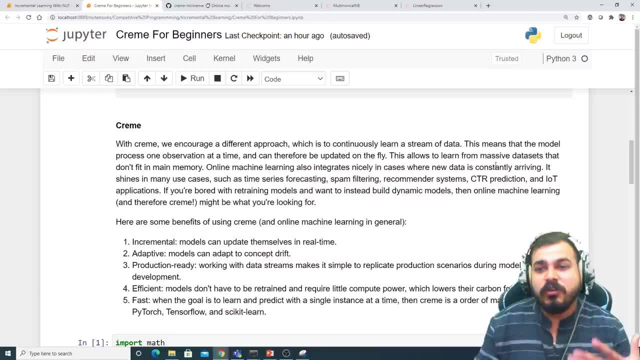 the main memory. So what does this say? that it allows you to train your model with one observation at a time. also, that is how it can be done in deep learning. I think you have heard of something called as batch mode. right in batch, you will be specifying some batch size because you will not be able to fit. 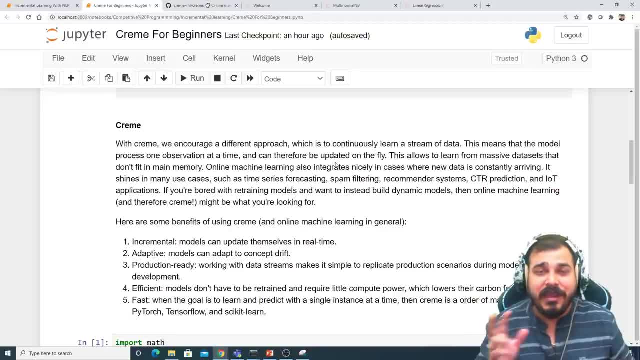 all your data set into the memory at the same time. so, over there again, you use different kind of optimizers, you use different kind of gradient descent, like stochastic gradient descent, and all this can make you confused. but, in short, what it says: that you can retrain your model with taking 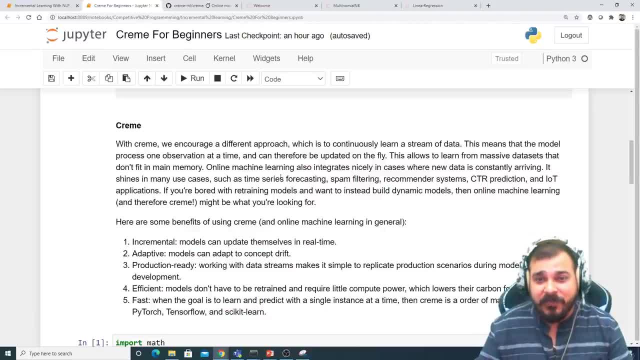 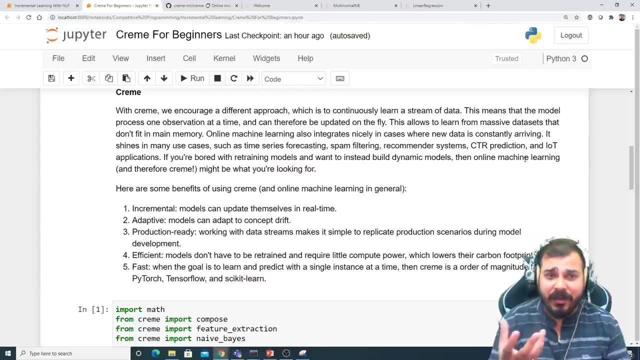 one observation at a time. okay, that is the most important thing. so online machine learning also integrates nicely in cases when new data is constantly arriving. now you may be thinking, guys, with respect to CREME, will we have all libraries like all algorithms, like how we have for a skill on? yes, guys, most of the algorithms are actually present in CREME libraries also. 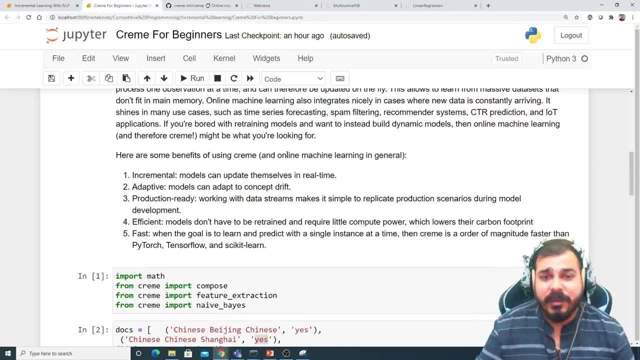 okay, so I'll try to show you too. here are some benefits of using CREME. uh, incremental model can update themselves in real time. suppose if, if the model is in the production also and continuously, data is actually coming, you can train it at that time. uh, it is. 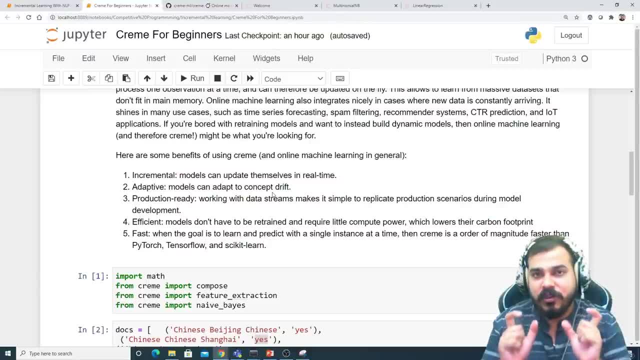 adaptive models can adapt to concept drift. this is what I was actually mainly focusing on: drift, machine learning, right. what does this basically say? this basically says that suppose I'm getting new data and my model starts performing badly at that time. I definitely have to see that. what that? 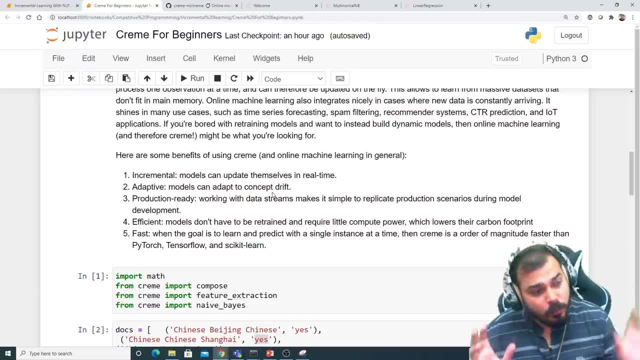 specific new data is, and I really want to just train my model with the new data on top of the old data that is already trained. I don't have to do the training from scratch, right? so that is also the thing that we are actually trying to focus over. 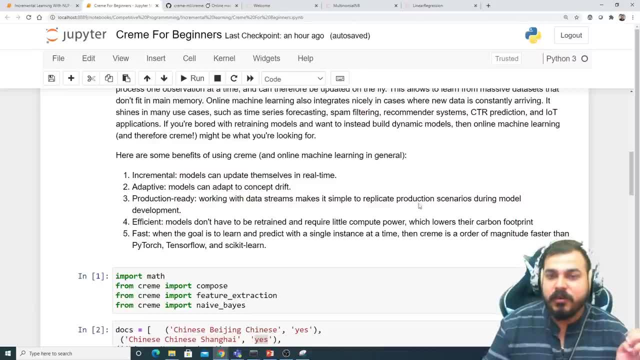 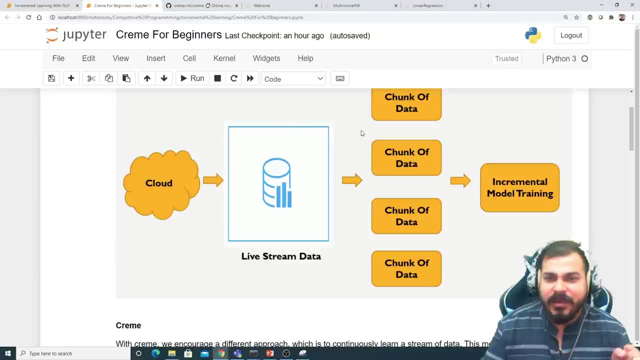 here it should be production ready. working with data streams make it simple to replicate production scenarios during model development, obviously. so this diagram that I have drawn. okay, suppose, if it is stored in the big data, I will be able to take this as a live stream, continuously take. 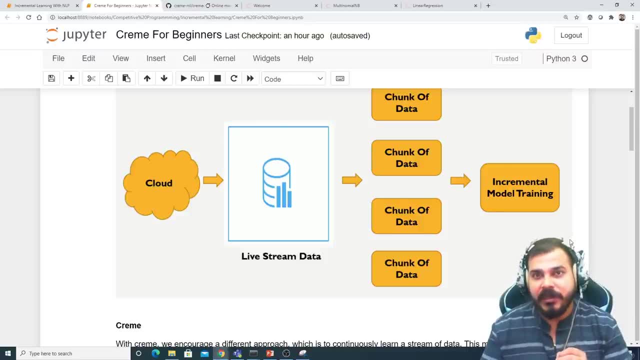 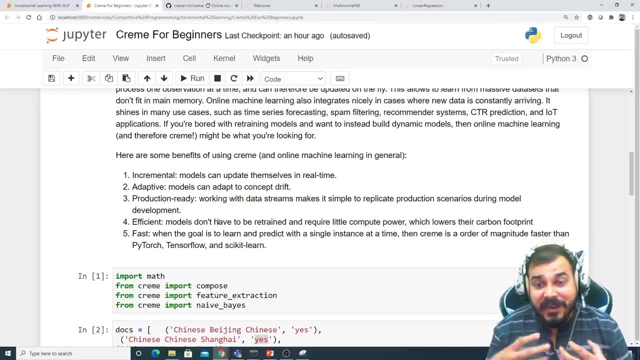 chunk of data, one observation at a time, and do the incremental training itself, right then, uh, it is efficient because, again, it it requires. it did not? the model did not be trained from the scratch. that is the most important thing. okay, it requires a little bit compute power. I'll also be 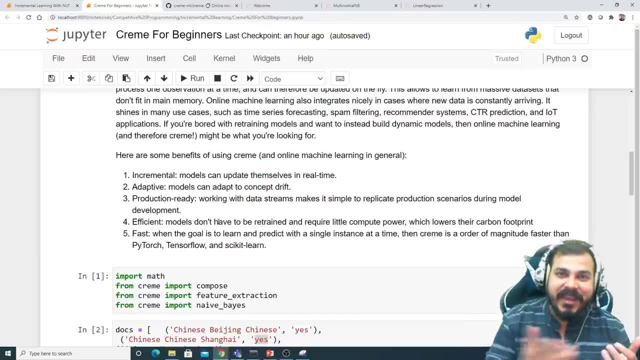 showing you the time stamp that they have given, like how much time it will take to do the retrain. uh, it has. Cramer library is very, very good. I think you should start using it. I've been, I've been actually exploring this particular library from past two to three months and finally I was 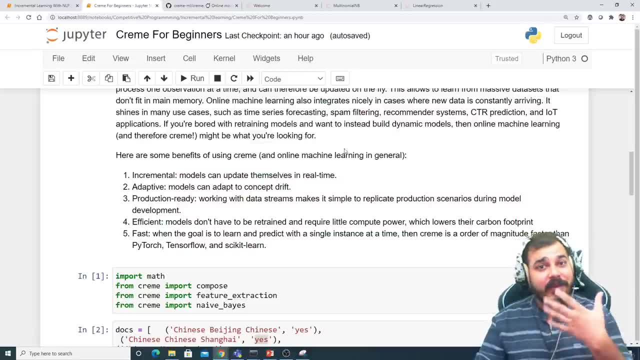 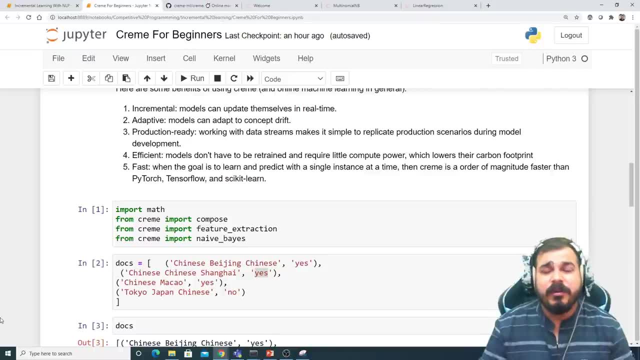 able to make this particular video, because this is one of the most wanted video, like it was requesting. so let's start and do this by taking some very good examples, some simple examples, so that you'll be able to understand. so, first of all, what I'm going to do is that, guys, we 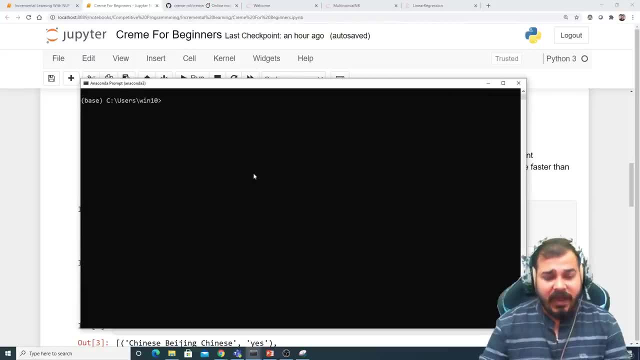 have to install crema library. so what I'm going to do, I'm going to activate databases, right, and then I'm going to go to. I just have to write tip: install creme. okay, you just have to write like this and always make sure that guys try to always create a new environment whenever you're working. 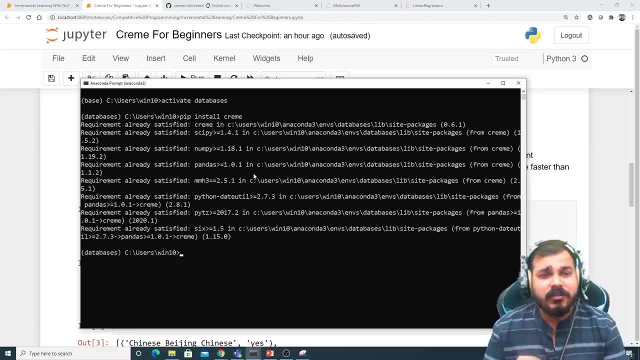 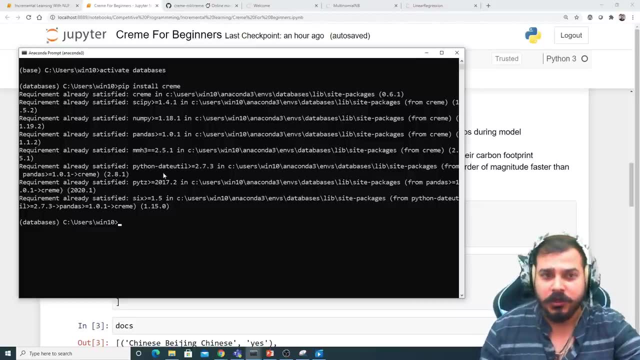 libraries, new techniques. that is always good. so once I install this, you'll be able to see that requirement is already satisfied. now, once the requirement is already satisfied over here, make sure that you also do the installation. guys, it will take hardly one minute. within one minute, the installation will happen. after that, what we are going to do is that I'm going to import some 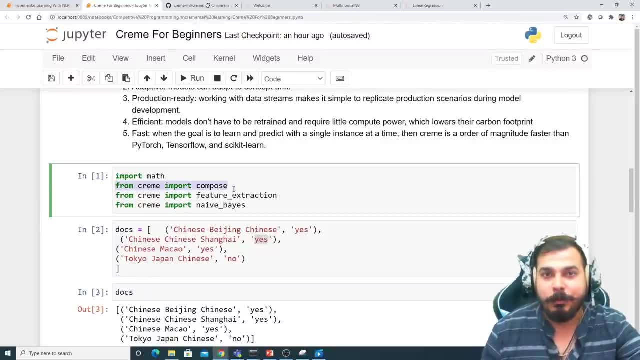 libraries like from creme import compose. this compose is basically used to create pipelines. okay, and in sklearn also, you have this libraries. you have libraries like feature extraction. you have libraries like all the machine learning algorithms and many more things. okay, only some of the machine learning algorithms, like xgboost is not present, I guess, but other than that you'll. 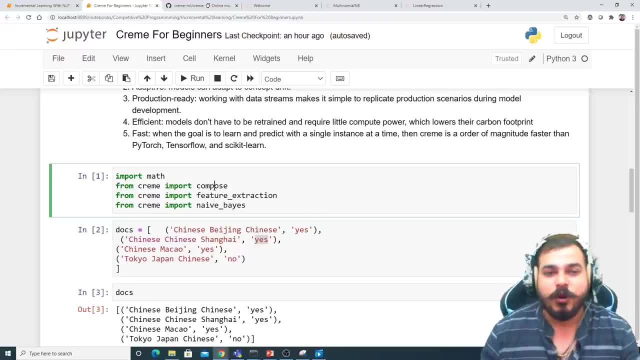 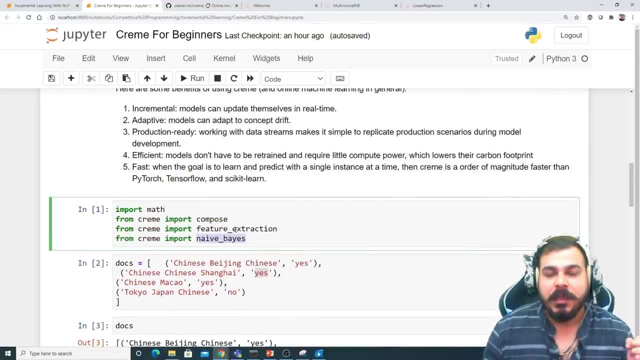 be able to find all the machine learning algorithms. so here I have imported compose, feature extraction and name bias. now let me just take a very simple example and always remember one thing, guys: whenever we are working with sklearn- right, whenever you're working with sklearn, at that time you usually 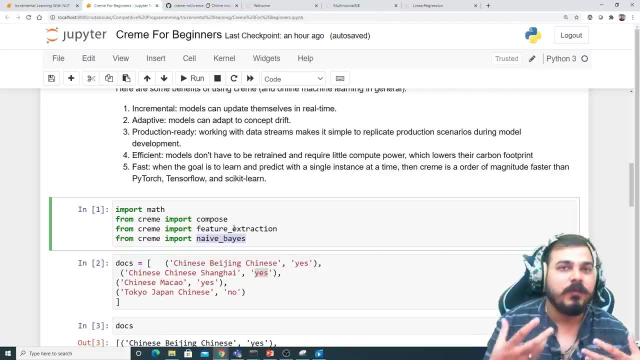 upload this particular data set inside data frames and then you convert that into independent and independent features and then you train your model with the sklearn machine learning libraries. but in case of creme, you have to keep all your independent and dependent features together in the form of tuples. okay, that is the most important thing that you should remember. okay, so in this, 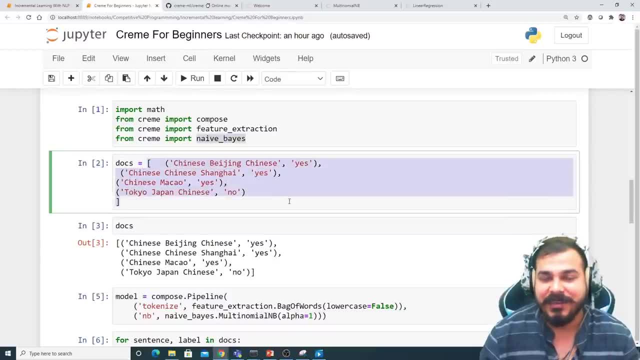 particular case. I have taken some list of text and this and I'll also be showing you after this. this is just a basic example. after this I'll try to show you how you can actually perform this in a data set also. right, so that particular example, I've actually taken this. 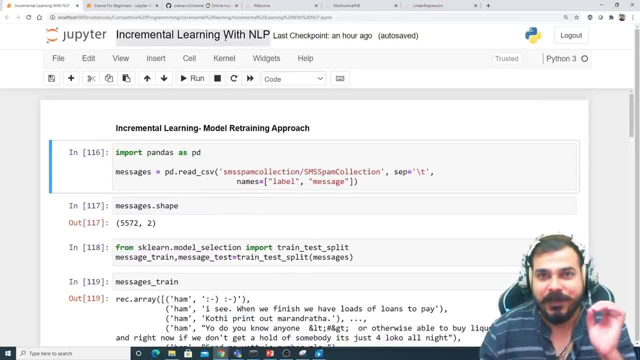 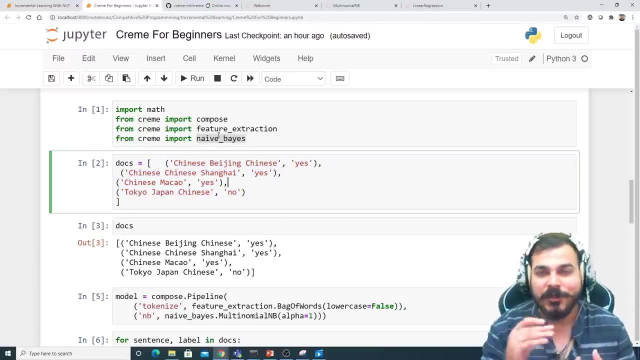 and here the first thing that we will be actually doing is with respect to nlp. okay, and in the upcoming videos I'll be showing you other algorithms also. so, with the nlp, what I'm going to do over here, I'm going to use multi-name bias. and one more thing that you have to remember, guys: 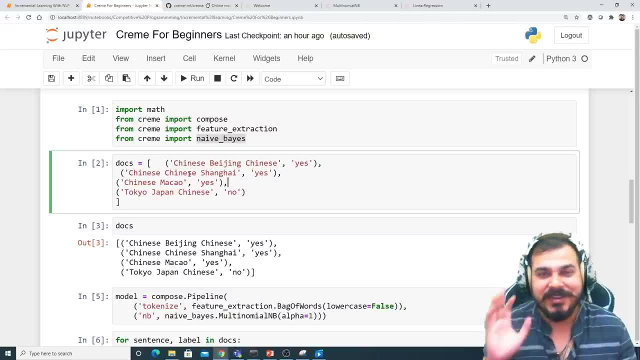 creme also works with garras. so there are a lot of videos, interesting videos, that I'll be showing you, which will be very, very helpful for you. now, suppose in this list- uh, this is all my independent feature text and this is my output, so here we are just trying to detect, like, uh, suppose if 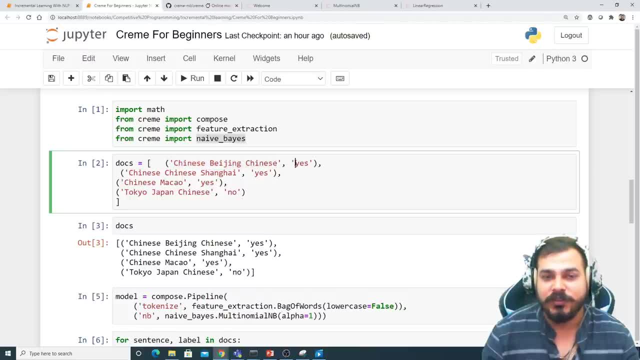 it is having uh words like Chinese, basing Chinese, I'm going to say yes. uh, if it is having Tokyo, Japan and Chinese like this combination, it is going to say no. and one more important thing about creme, guys, suppose I, in this particular uh example, I just have two texts right, two outputs. 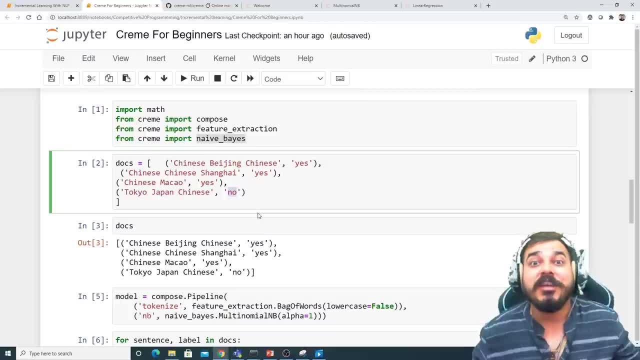 like yes and no. with the help of creme, tomorrow, if you have a new category also, you will be able to train your model and I'll show you in this particular example also. okay, so this is an independent and the dependent feature are in the form of tuple. so this is basically the list of 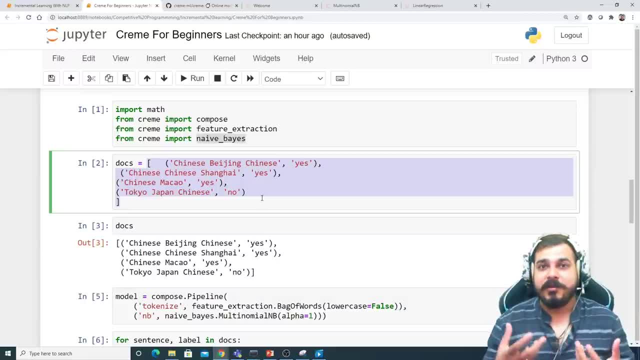 tuple. okay, that is the thing. that is what the creme libraries basically accept as an input and always remember the first parameter will be the sentences and the second will be the labels. okay, so suppose I have created this Docs and this is basically my Docs. this is my input. features in: 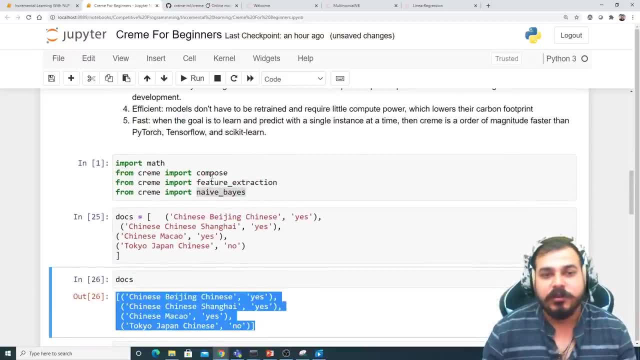 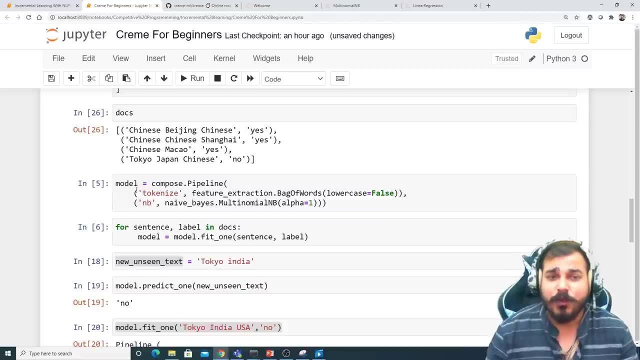 which I have to train my model. now, as I told you, I have gone to use this compose to create pipelines. pipelines basically means I've created a lot of videos regarding pipelines, right suppose? I want one uh feature like standard scalar, I want like tokenize, I want like a name bias. this is basically the name of the pipeline and I can put any number of pipelines. 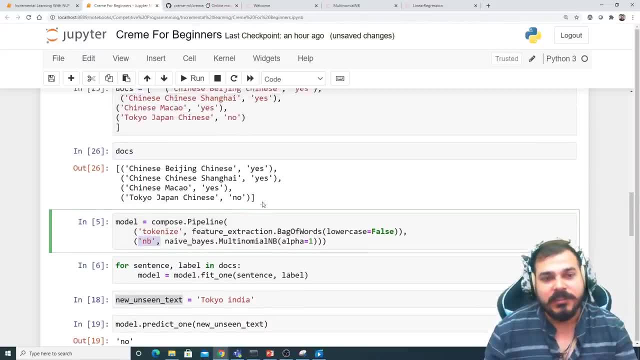 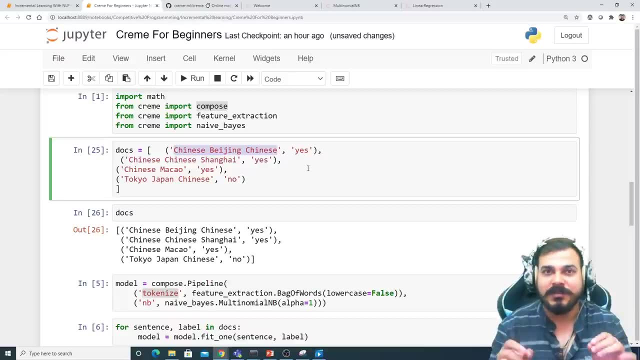 like this. right, I can use standard scalar also and all. now, first I'm actually going to do the tokenizer in tokenizer. you know that we will be converting this words in case of nlp, we will be converting this words into bag of words, into tf, idf and all. so how do we do that from this? 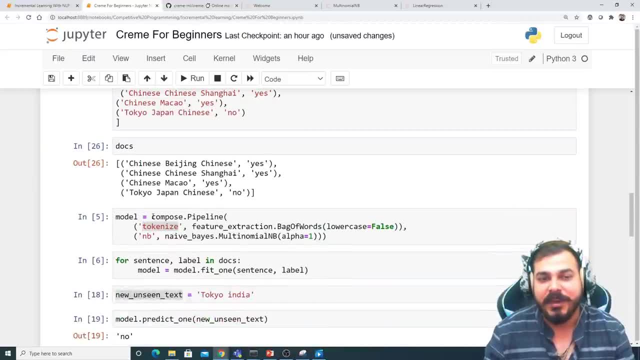 particular library which is called a feature extraction. so here you can see that I'm creating compose dot pipeline. pipeline actually helps you to create, like, after one step, what is the next step that will happen? so in this case, after tokenizer, we are just going to apply multinomial new bias. you can also add standard scalar, but standard scalar, I think, will not. 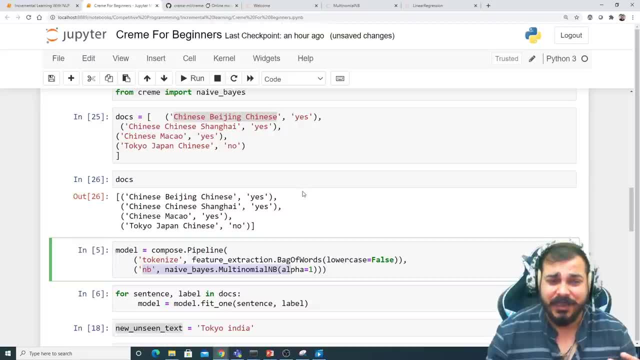 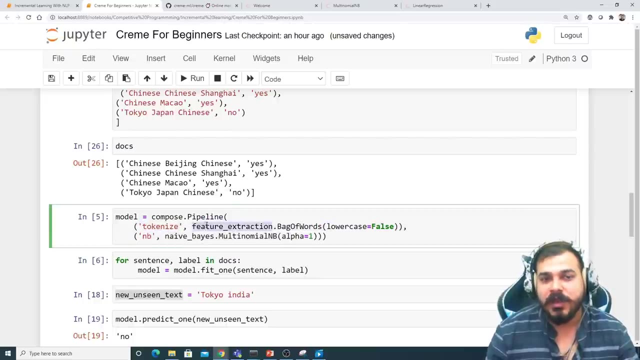 require in this particular case, because this is completely a text pre-processing technique. but when I'm doing some algorithm like logistic or some ensemble techniques- not ensemble logistic or linear regression- at that time I'll be using standard scalar. so here in my first pipeline I'm going to use standard scalar and this tokenize is doing the bag of words: considering, by making the 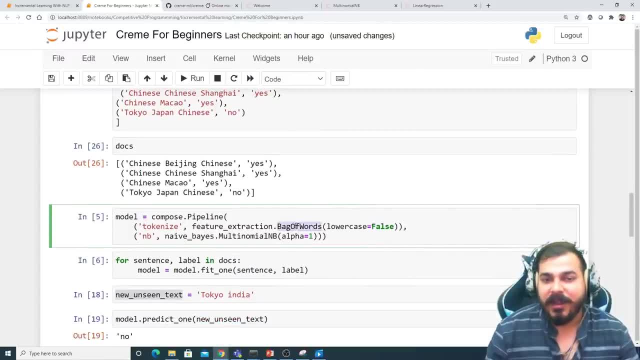 lower case as false. that basically means it is not compensated that we need to have a lower case. okay, now this bag of words. let us see what all options we have other than that. so if I see over here, there is options like aggregate. there's bag of words, there's target tag, there's tf, idf, right. 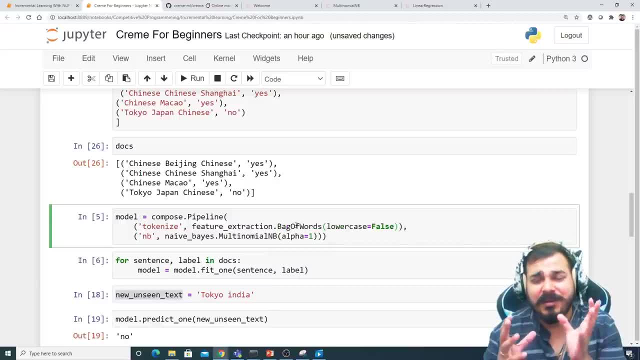 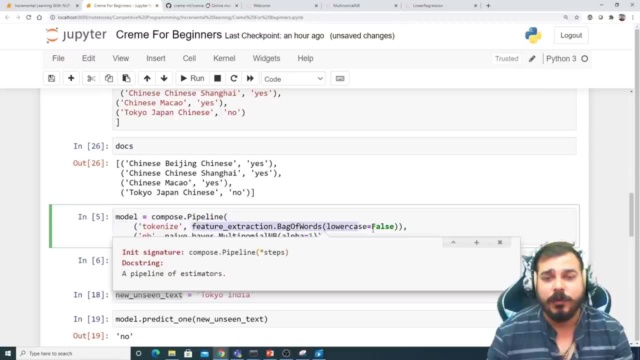 there is also called as vectorize. so right now I'm just going to use the bag of words, because we are doing a simple classification problem with respect to text, and over here you can also check out all the what is actually present over here. so if I, if I just copy this and if I make a cell on top of it, 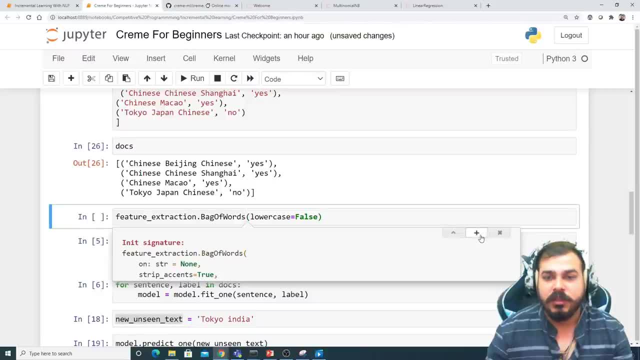 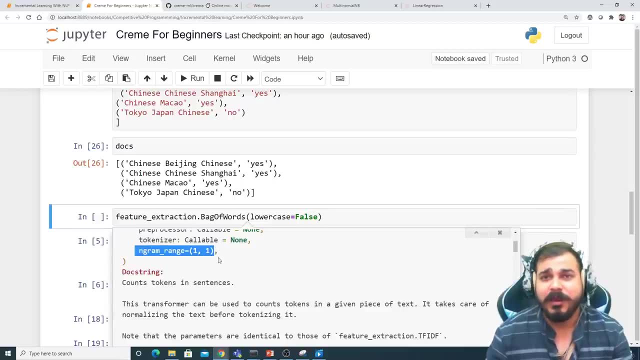 so if I go and press shift tab you'll be able to see all the parameters over here. so lowercase is very basically true or not, fire false. all this ng gram. by default it is one comma one. you can change it to two comma one, right three comma one. that is up to you. so this is basically the example that I 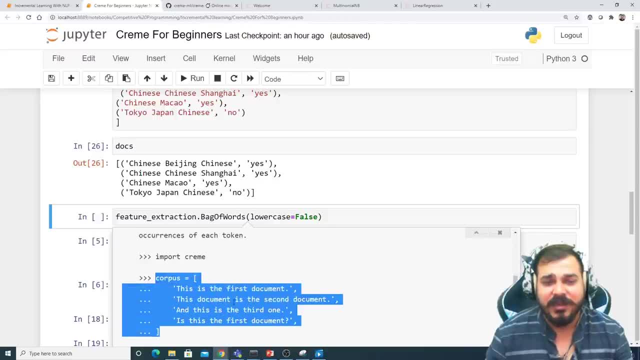 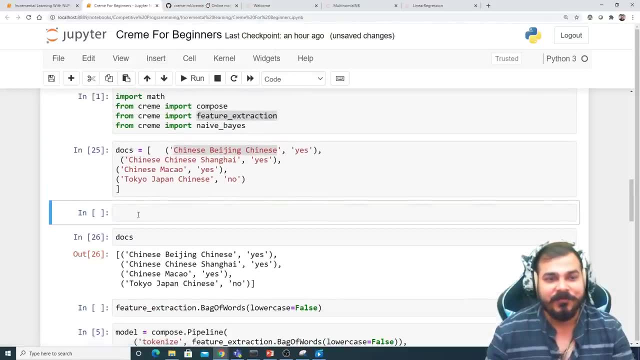 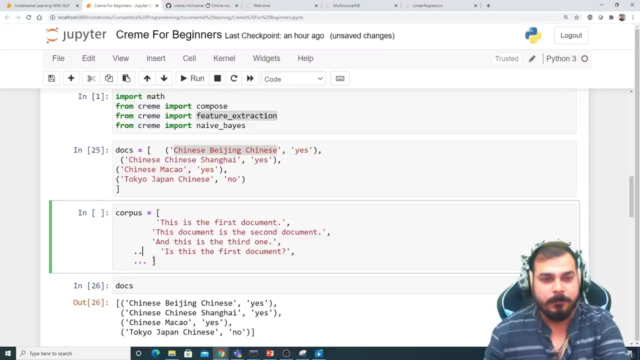 was actually taking right. so suppose, if I take this as my corpus, right, and if I try to convert this into back efforts, let me take this example also so that you will be able to understand very much easily. okay, so I'm going to just take this, I'm going to remove this, okay, okay, and, as I said, that I'll just go. 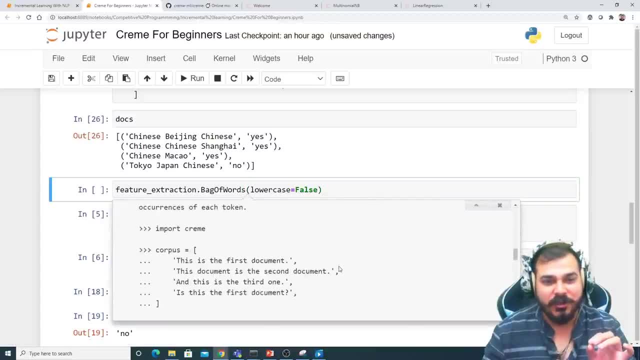 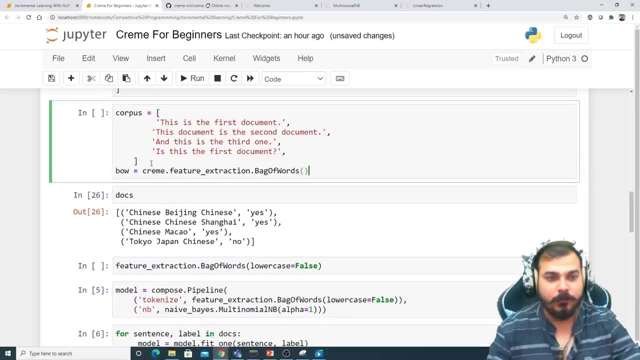 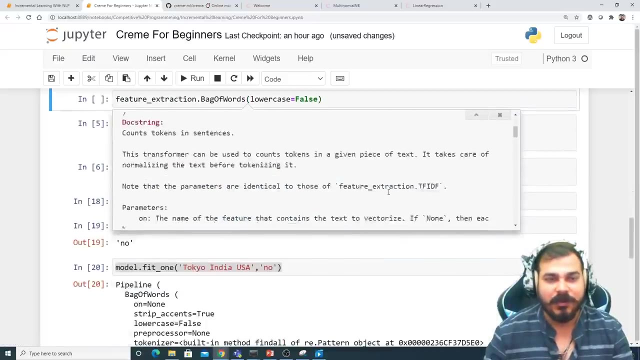 and check this example just to show you guys again, in this project you need not do it, so I'm just going to use this one, okay, bow. uh, I'm going to paste it over here and again I'm going to, and again, all these materials will be given to you guys in the GitHub and just check it out. uh, I'm. 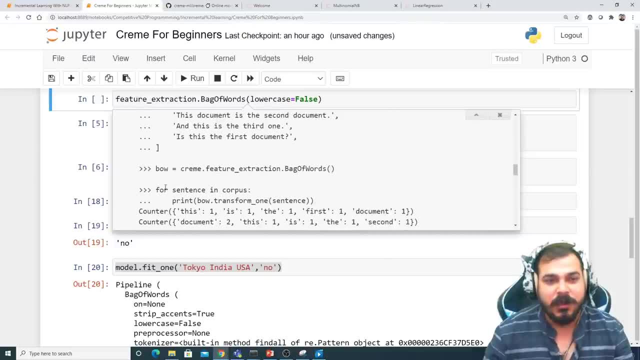 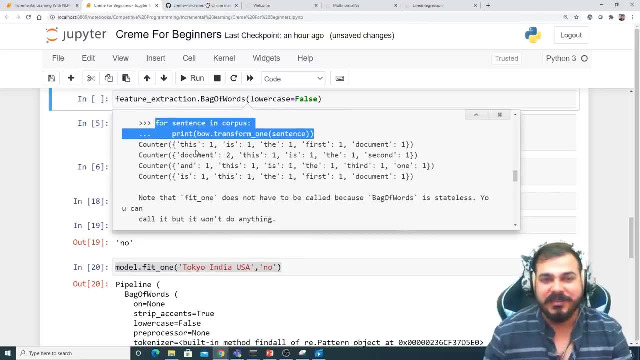 just making your work a little bit easier to make you understand how things work. uh, after doing this, I can use a for loop and I can print like this, so you'll be able to see that we'll get the output something like this: this will be given as one. uh, like that kind of you know, bag of words is simple. 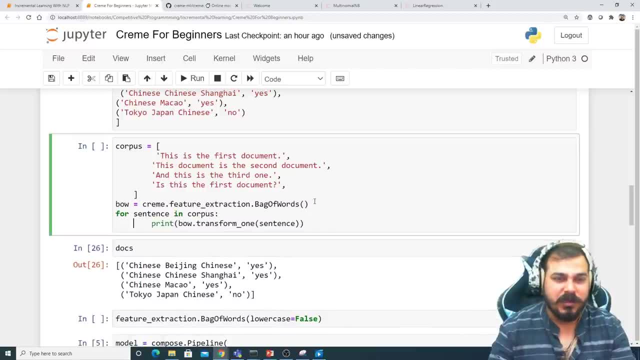 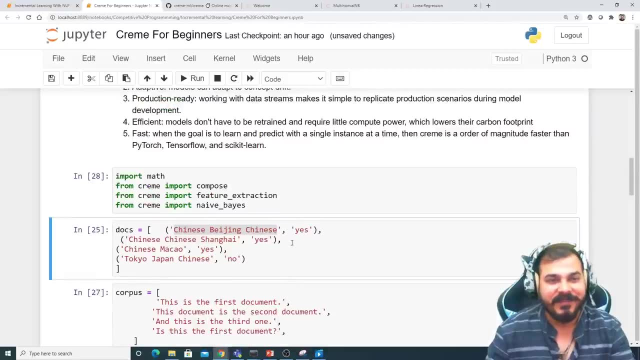 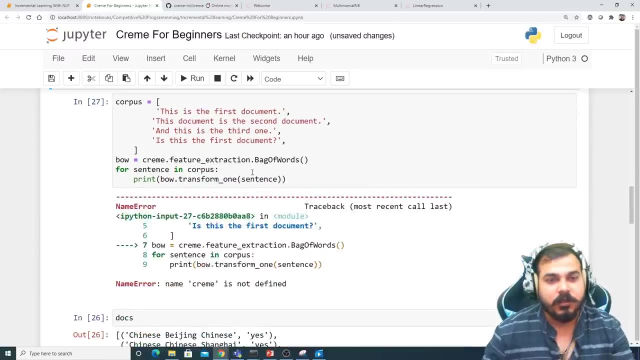 right, you will basically be converting a text into uh, vectors. so here you have. okay, I did not import, why? okay, let me just import cream also. so we will be requiring credit, right, perfect, so let me just execute this now. here you'll be able to see that this is given the vector as one is one, the one. 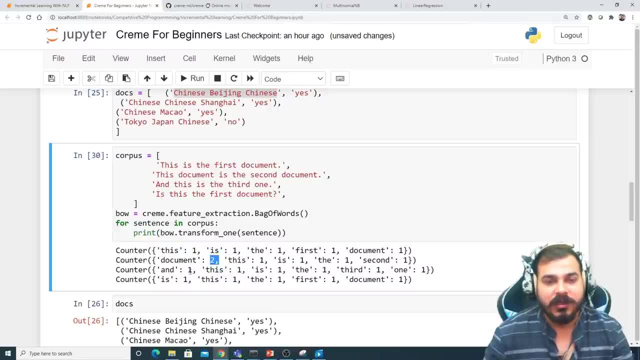 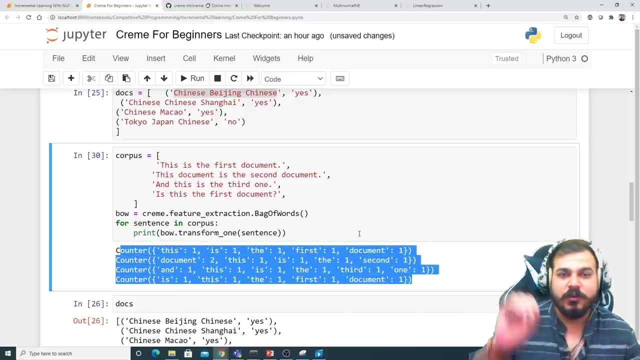 first, one document, one. this document is two. then here you can see all the same, like how bag of words work. this is just nothing but the counter, simple counter with respect to bag of words. if you don't know about that, check my NLP playlist, guys, and suppose if I convert this into TF, IDF. 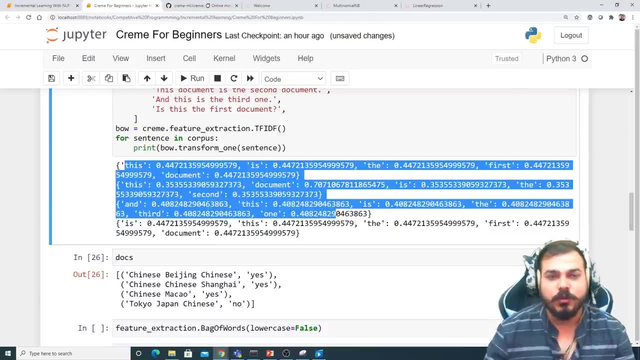 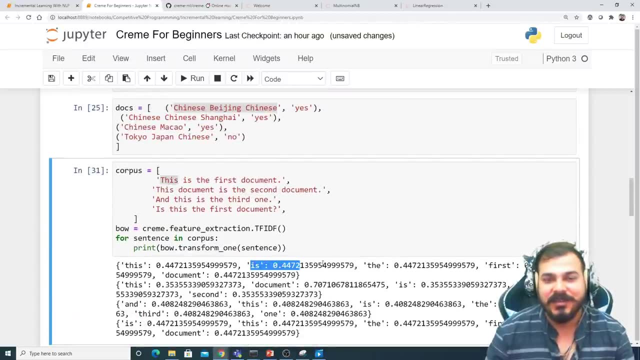 then you will be able to see that how these words are actually getting converted into vectors. but this is giving an idea, right? this, this is basically given the vector. this one is given the vector, this one. right, it is pretty much simple, pretty much amazing itself. okay, now let's go back over here. 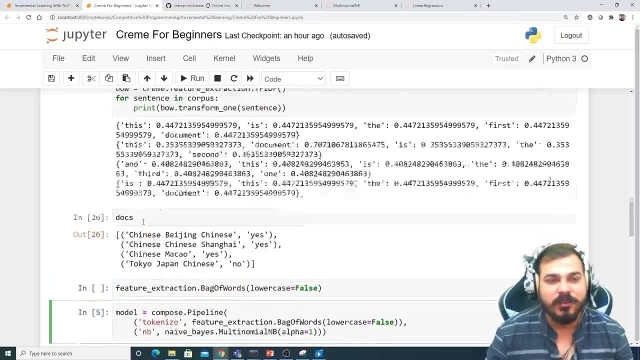 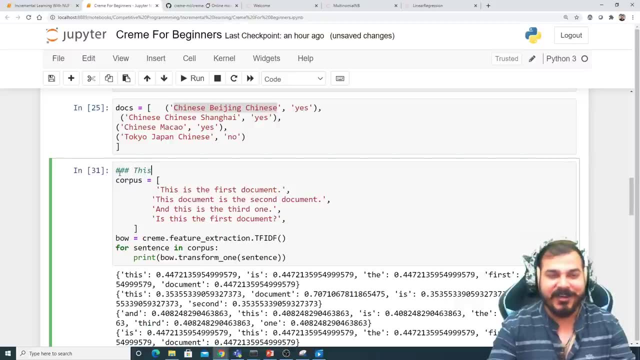 so what I'm going to do is that I'm going to create, I'm just going to remove all these things. so that you don't get, I'll write it over here. this is just an example, okay, so that you should not get confused, guys. this is just an 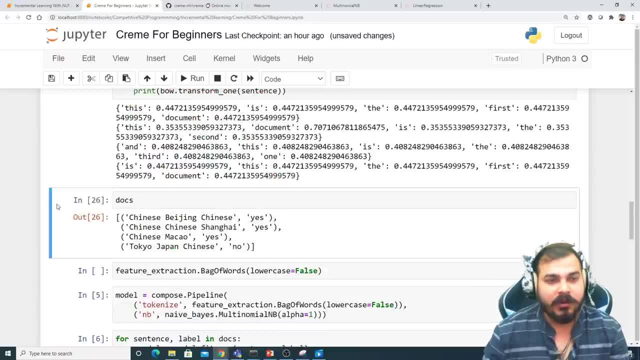 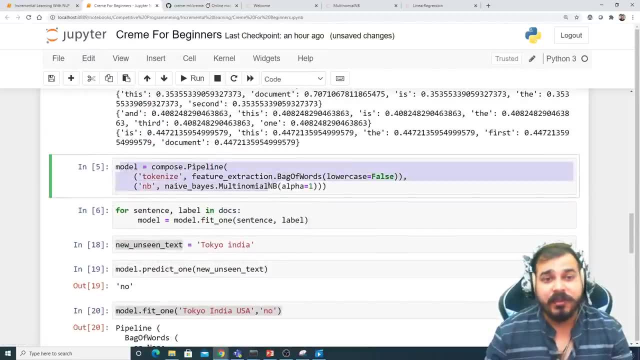 example: okay, perfect, uh, I'll remove this because I don't require this and this, right. so again, just to make your work easier. so here I'm actually create a pipeline. in the first pipeline we are going to do the. the pipeline name is tokenized. there we are actually performing bag. 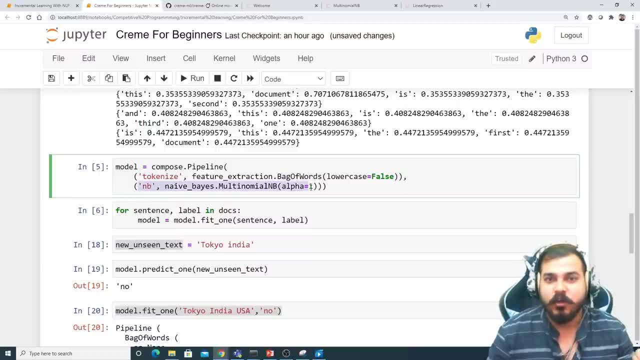 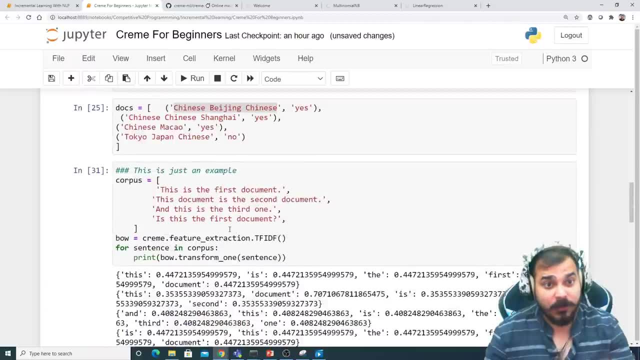 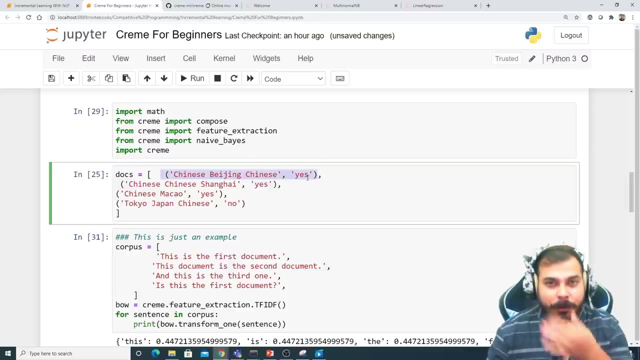 of words. you can also perform DF idea. then I'm actually applying multinomial name. bias with Alpha is equal to one. okay, so once I execute this, this is basically my model. now you understand one thing, guys. uh, my Docs is basically having the tuple effect of two things. one is your sentence and your label. okay, so I'm just going to give a temporary. 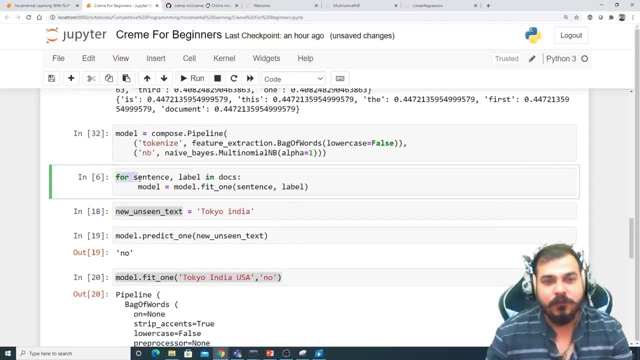 name because I I really want to iterate through this. so I'm putting a for loop for sentence comma label in Docs. so sentence I will be. I will be using this as my input feature and label will basically be my output feature now when I am iterating to this inside the model. 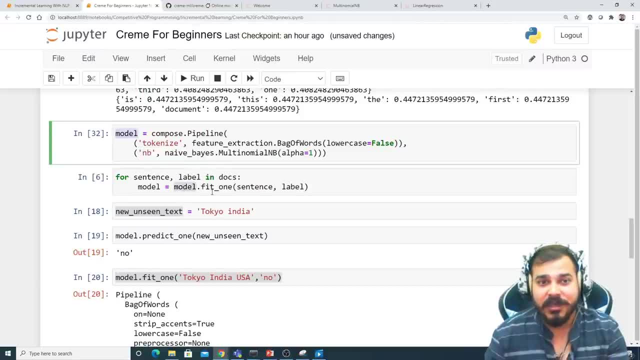 inside this particular model, which is created from crema library, you have one function which is called As ус, fit underscore one, so fit underscore one will be taking one. with the last dot there is got a one then, perfectly normal. so we'll stick with this into our space list of options and we'll go with. Oh, this means that the logo will not be a default, so a bullet point is: 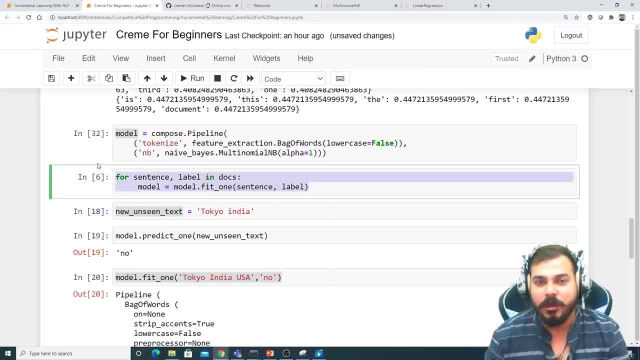 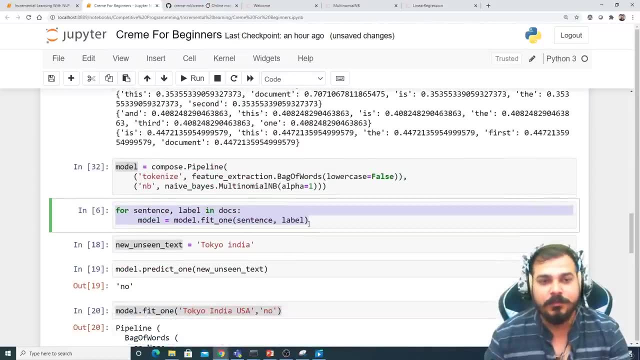 be taking one sentence at a time, one label at a time, and it will be training the model. so, like this, we will be training all the documented, all the documents that are present inside this docs. okay, pretty much simple, so i will try to execute this. you'll be able to see, guys. 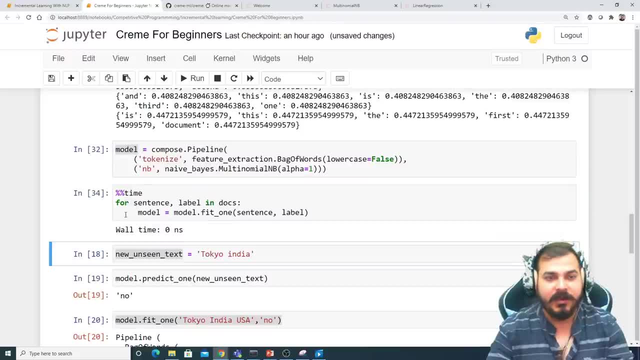 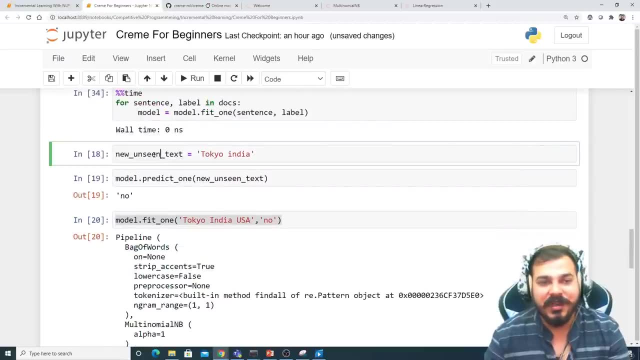 when i am actually training. also, right, if i write time, you'll be able to see hardly it is taking any time, right? so the training has happened. now what you will do is that suppose the news unseen text is like this: tokyo india, okay, tokyo india. if i execute it. and now if i write model dot predict. 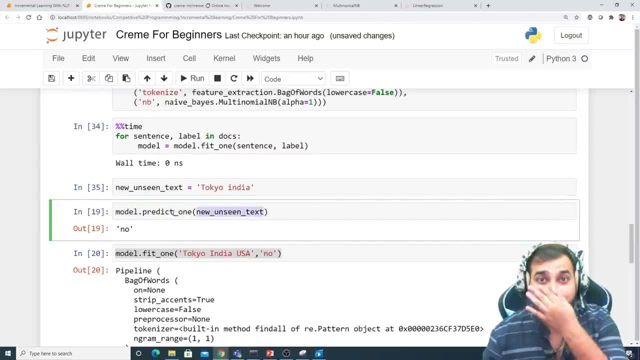 underscore one on new unseen text. okay, suppose, if you have multiple text, there is a again a function which is called as predict many. okay, if you have multiple text, if you just have one text, you can use predict one, and if i execute this, you'll be able to see. the answer is no. the reason why answer. 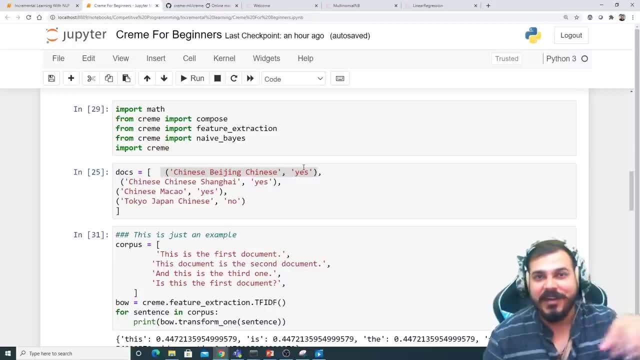 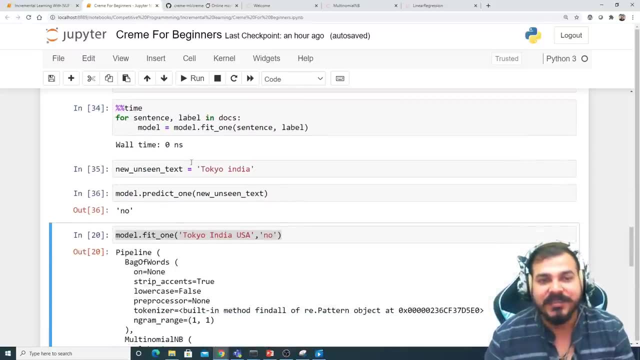 came as no. now again, you see that, guys, yes, we did not convert as zeros and ones, we did not do the direct conversion, but we gave, just like that specific label. now why this answer has come as no? because you can see that tokyo was basically present in the no category. india is not present over there, right? so definitely. 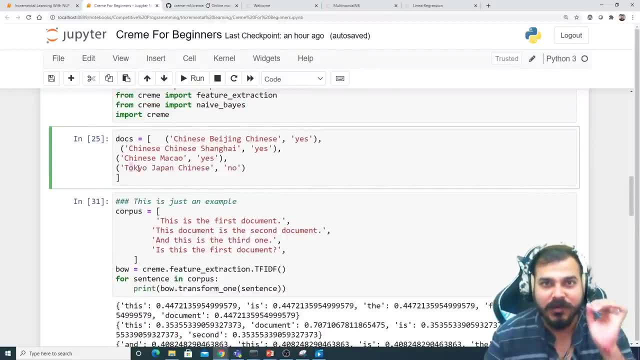 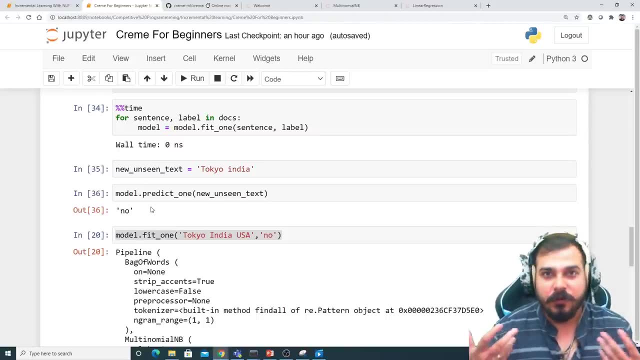 if i'm using bag of words, that value will be zero, but wherever tokyo was one, it is basically considering as no. now you may be thinking: okay, krish, fine, that is absolutely perfect, as you told that we can add a new category. just show us that particular example now. in in the future, you'll be. 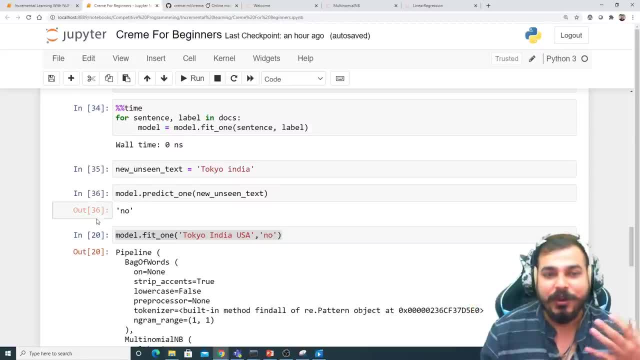 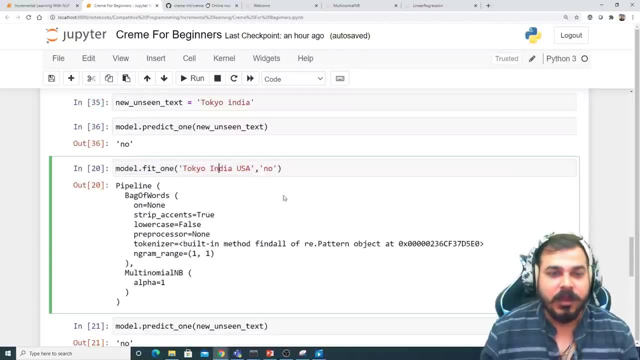 having new text. you can add a new category. just show us that particular example now. in in the future, you'll be having new text, new category, right? how do you do that? how do you train a new data into this? so for this, let's see, uh, what are things we can actually do now, here you can see guys, uh, what i'm doing is that i am i'll. 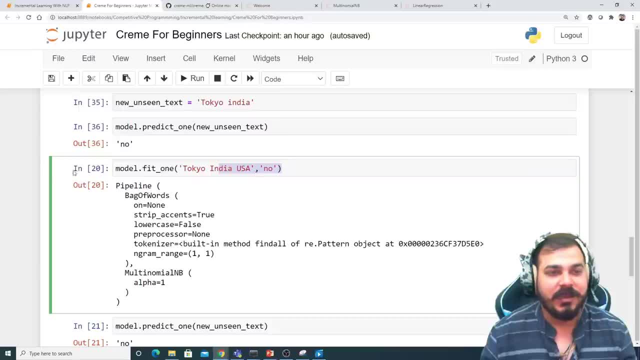 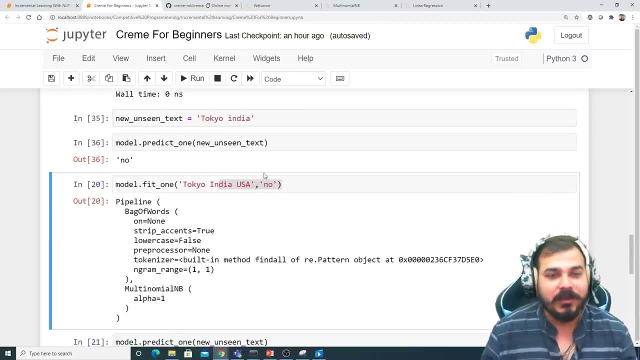 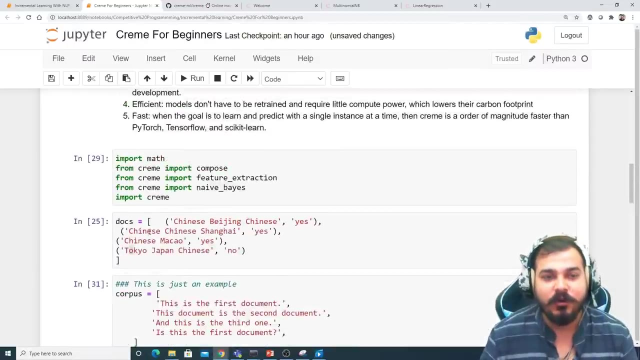 just remove this. okay, just i'll, because i really want to show you this is the most interesting part, okay, okay, now suppose i say that i don't find india and usa over there. see the words, guys. i don't say find, i don't find india, usa anywhere. now suppose i really want to create a third category, because 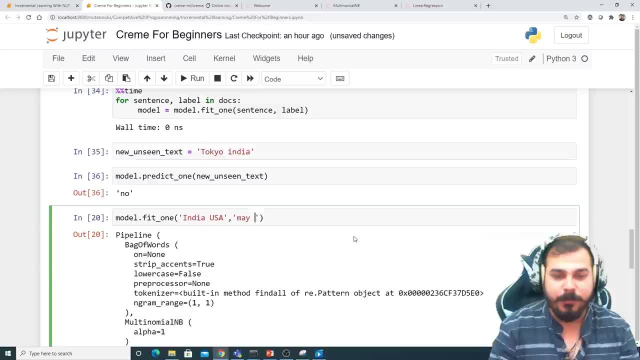 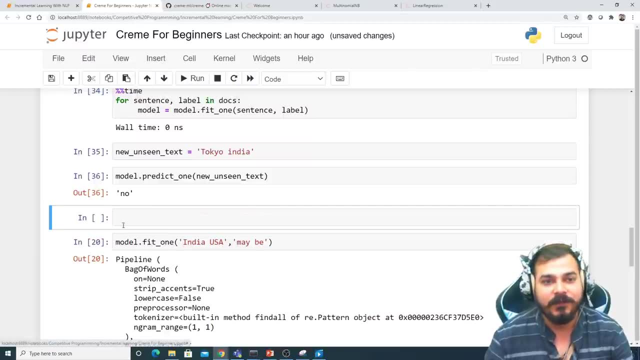 like neutral, or yes or no, or it may be maybe. okay, suppose this is my third category. this is my new text, okay, so what i'll do is that i have- i'll just write it over here- training on a new data and new category. see, i'm. 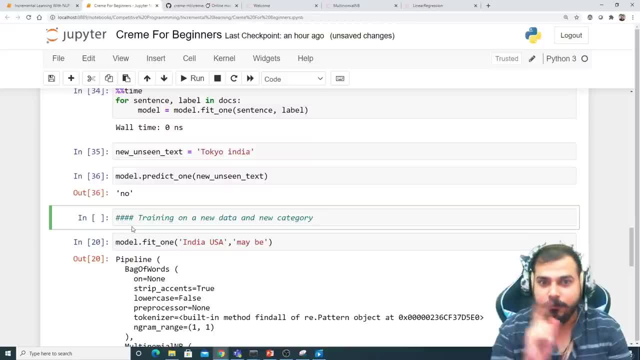 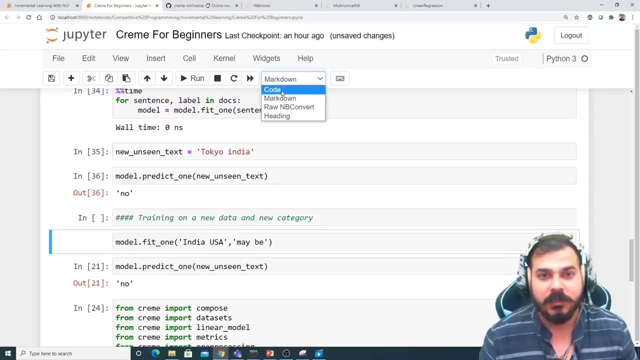 doing both okay. new data and new category also. i'm doing it both okay. i'm just not doing with respect to only new data. new data: it is possible with the same uh, with the same label like yes or no, but here i'm training on a new data with a new category. just a second, guys. so i'll make it. 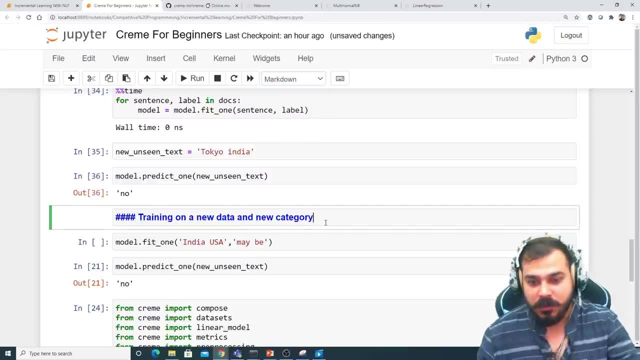 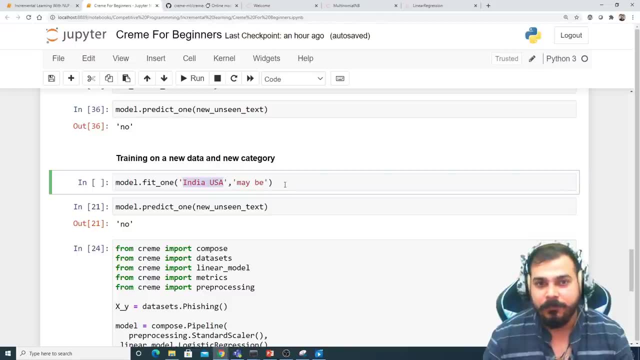 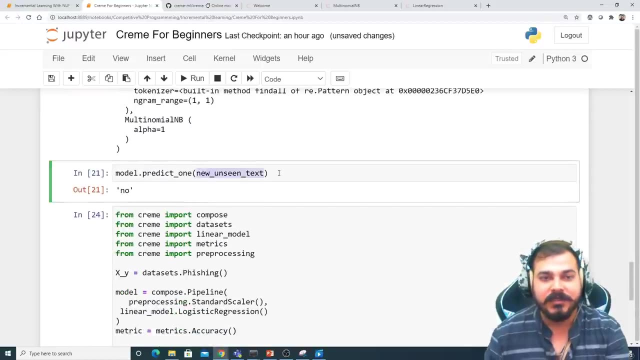 as code and this i'm going to make it as markdown. guys, this is important, just see this. so here i have written fit underscore one: india, usa- and i have written maybe okay, and now i'll execute this. okay, i've executed this. now suppose my unseen data is something like this. i'm going to just write it. 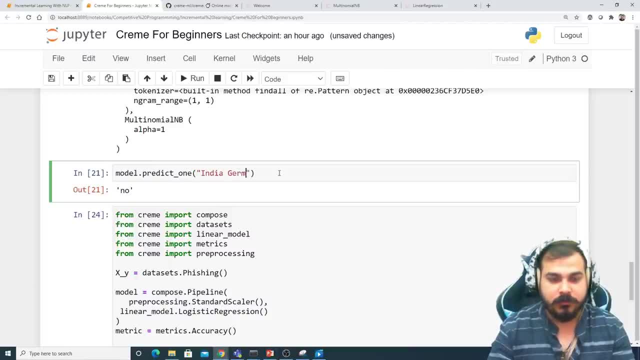 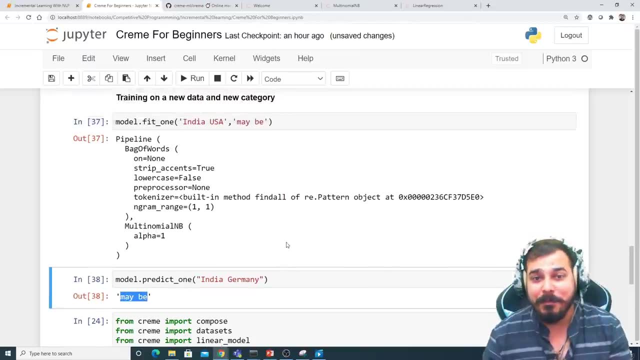 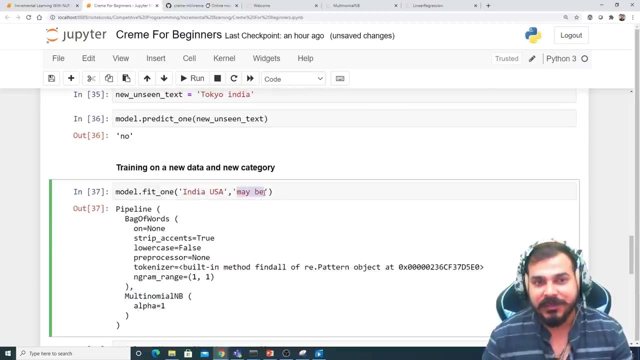 down over here as india, germany. i don't have germany over there and if i try to execute this, you are able to see that now it is being able to predict, maybe initially understand my model that was initially trained- was not trained on this, maybe output class, but just by using this fit1. 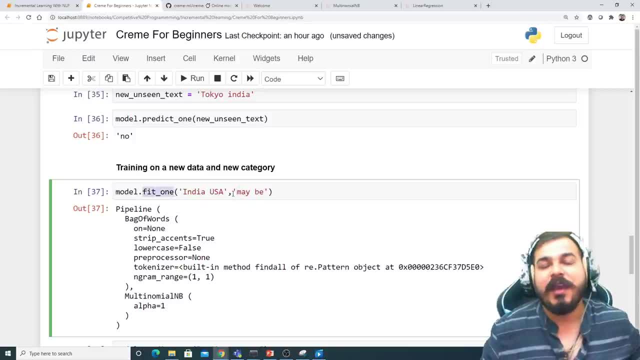 method. i will be able to train this, and i will be able to train this, and i will be able to train this. now, suppose, if you have many, many sentences, also, you can loop inside that and you can use fit one, fit one, fit, one and again, guys, uh, with respect to each and every sentence, you'll be able to do it. 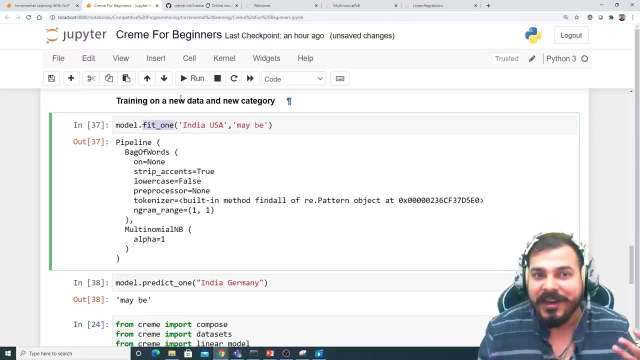 right now. what is the main thing that is actually happening over here? you're training on a new data and you're training on a new category. like that, any number of categories may be taken and yes to sometimes to get reflected. sometimes you require some good amount of data, but again, 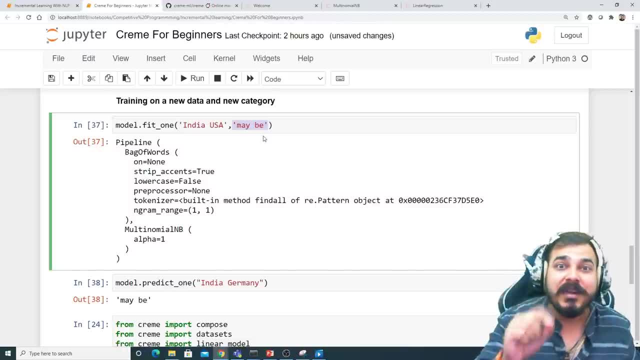 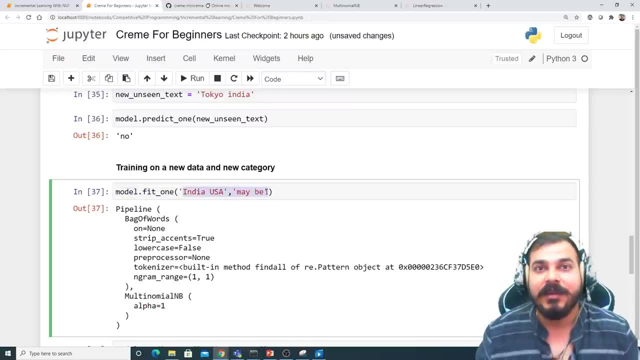 what is the thing that is happening over here? here the incremental training is happening because, after my model is getting trained, any new data that comes in the live stream i can train with that. and tomorrow suddenly i have a plan that i may have a new category in my data set. 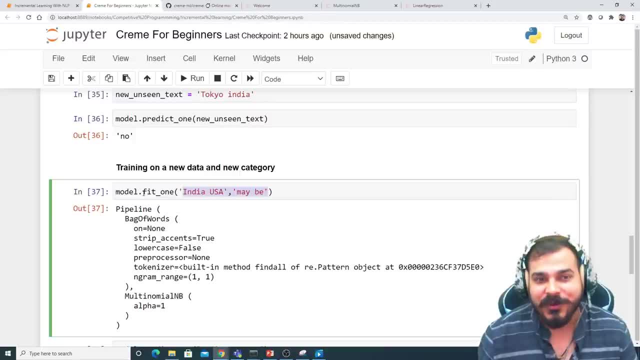 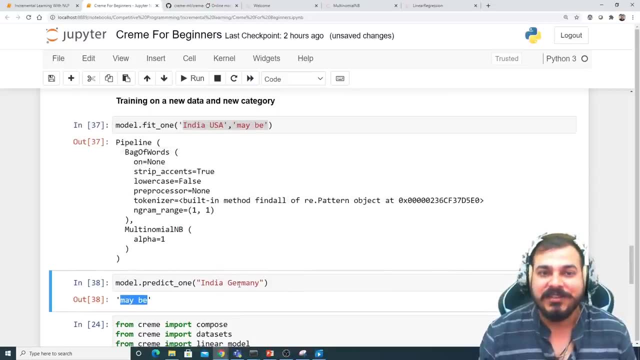 i may directly train it by the use of fit one method. so here you can see, by using fit one and by using the predict one, you are able to get the new category. and again, here i just use india and germany as my next keyword. right, right, i hope you are able to. 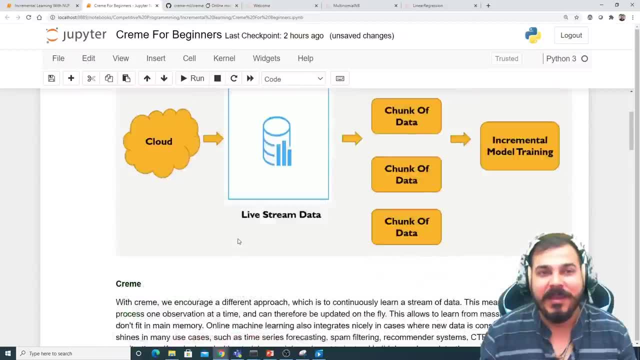 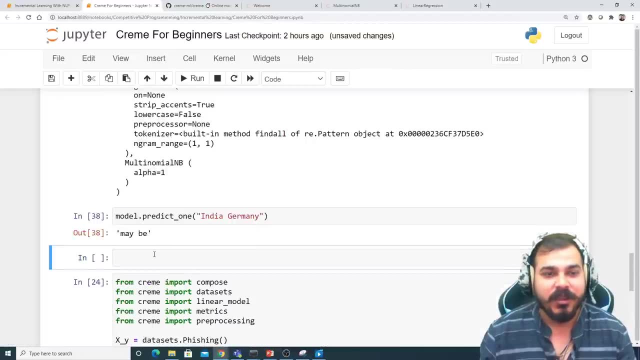 understand this, guys. so this was one example of nlp. uh, with respect to this again. uh, i'll will also show you the logistic regression which i have actually created over here. okay, this is just my logistic regression- creme with logistic regression, but i really want to show you and 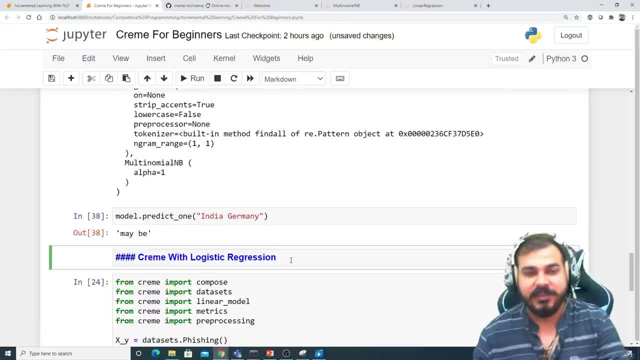 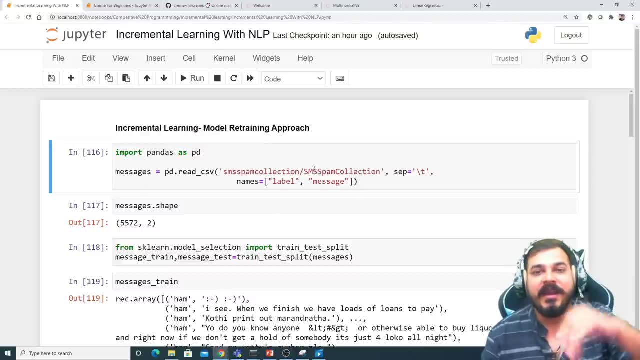 complete bigger problem statement. this was a very small data set. right, this was a very, very small data set. now let me just go with incrementing model retraining approach with a huge data set like spam and ham. okay, like spam and ham. so here you have: import pandas, spd. i'm reading some data: 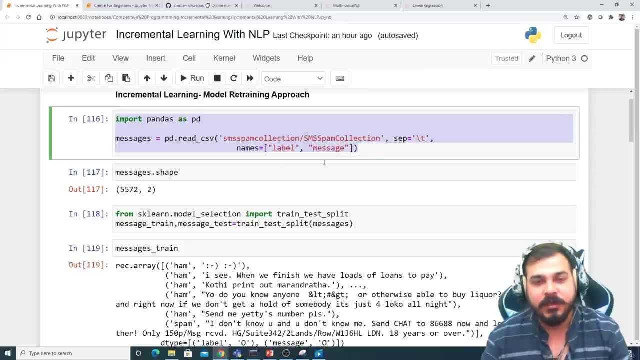 set over here. this data set will be given to you guys again in the github. so i've just used some separator slash t and here you have names, labels and messages. so i think i have downloaded this message, this data set, from uci uh website. so once i execute this, you'll be able to see that in. 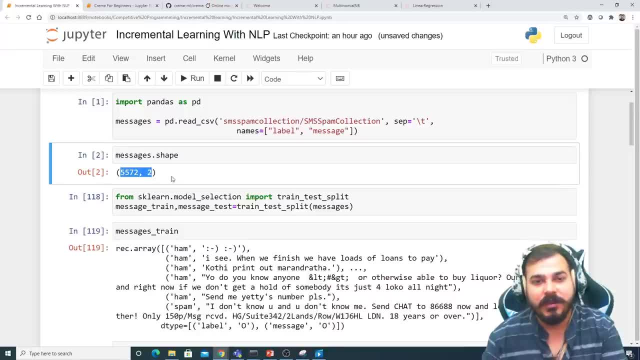 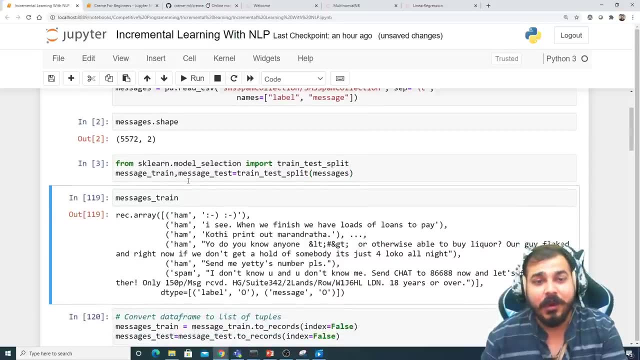 messageship: i have five, five, seven, two comma, two right. so i'm here using a skill on model selection to do the train test split, because obviously we're required to do the train test split now inside the strain test plates. i'm not doing x train, x test, y train and y test. 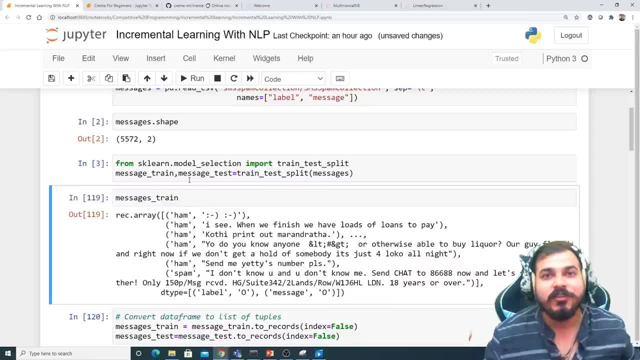 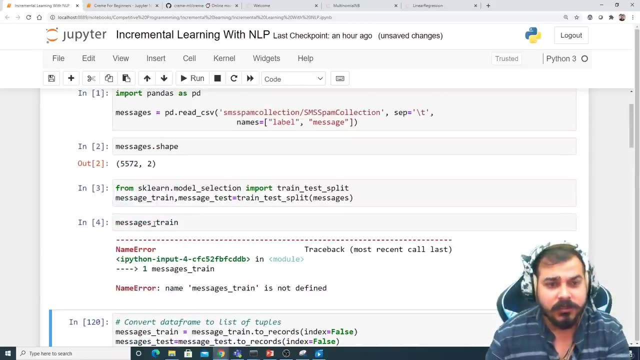 but instead i am doing train and test because i want to combine those uh training, uh input sentence and the label in the form of tuples. right, that is the first requirement with respect to creme. so here we have a message under to train. uh, did i not execute this messages? 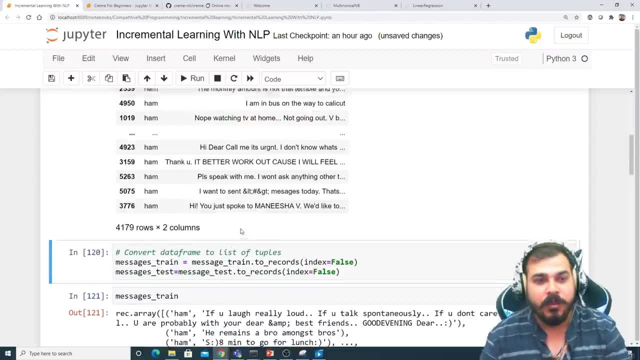 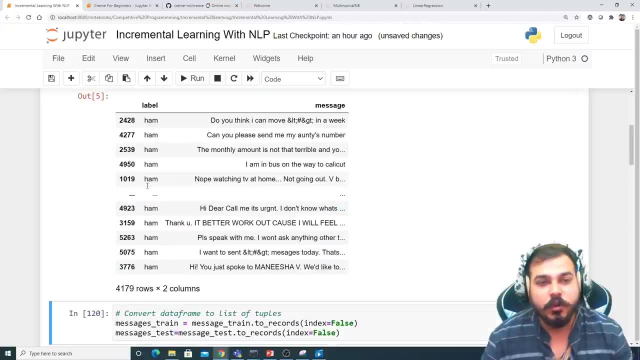 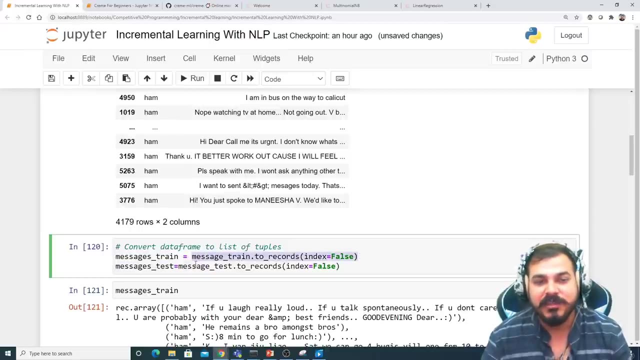 underscore train, so it should be message underscore train. okay, so this is basically my message underscore train. okay, and now what i'm doing is now, uh, this message underscore train. i am actually now converting this into two records. when i convert this into two records with index is equal to false. this will convert into a list or a list of tuples. so here you can see we will be. 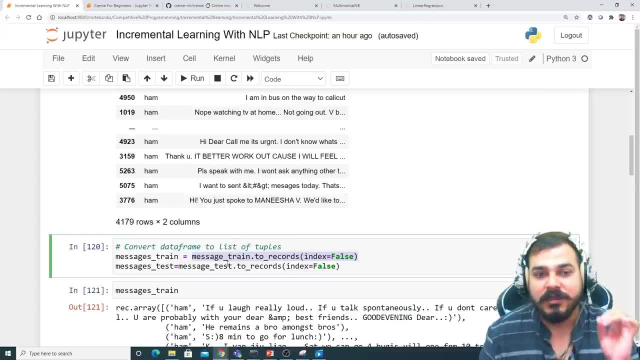 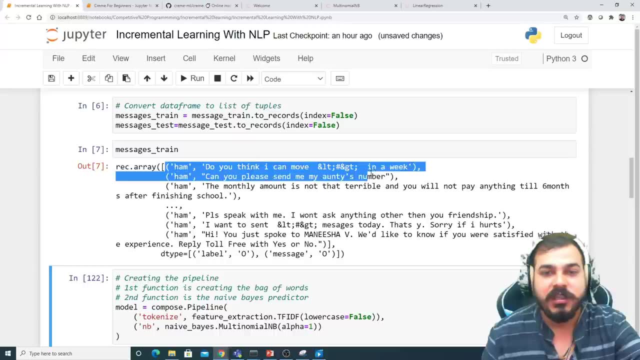 able to convert the data frame to a list of tuples. so i am trying to convert this for my training data set, also for my test data set. so if i execute this and if i now see my message train here you will be able to see the list of list of data, list of tuples. so here you have. first you have ham, that is your. 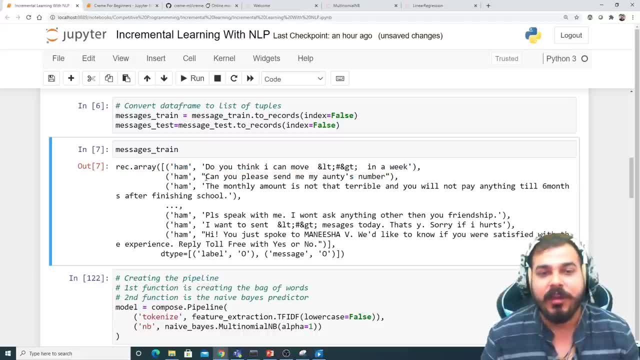 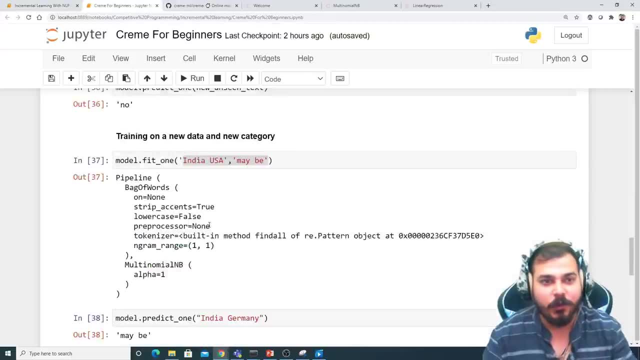 output feature, then you have a sentence, then you have, then you have your output sentence, so something like this. similarly, i have done it for the messages underscore: test perfect. that is the first requirement. as i said that over here we need to convert this into tuples. that was the first. 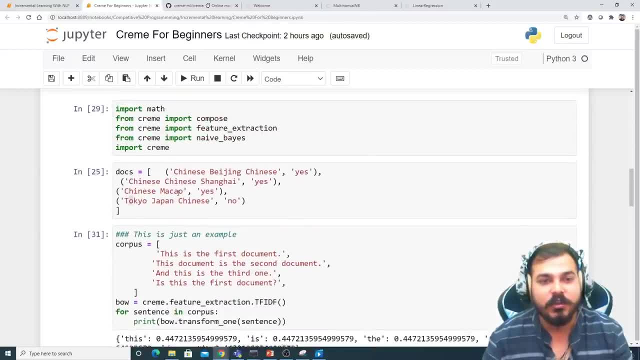 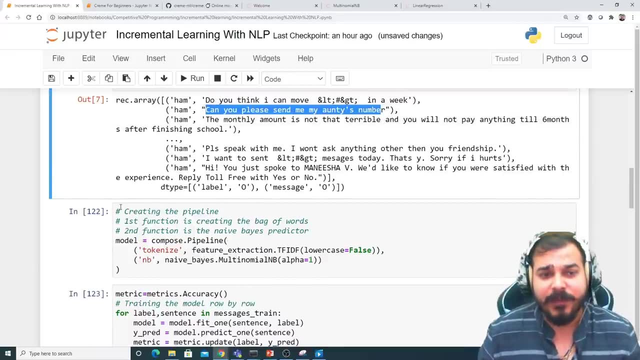 requirement that i told you over here also right, so we have converted this into tuples. so this, this whole data, is basically in the form of tuples now. now, obviously, we will be creating the pipeline. the first pipeline is basically to create the bag of words. so here, in this case, i have taken tf, idf. 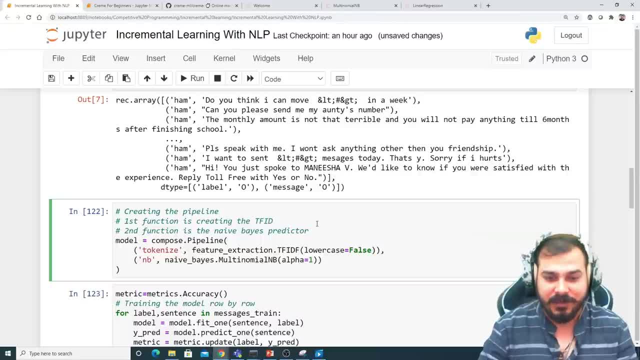 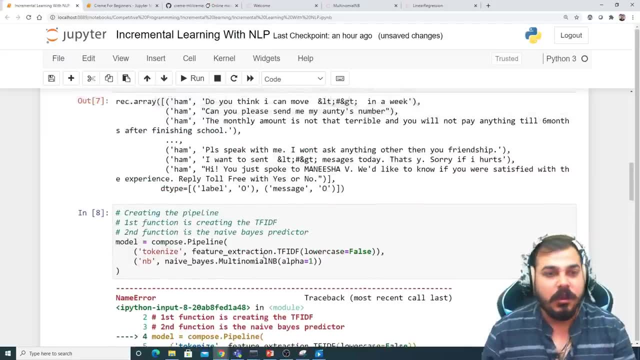 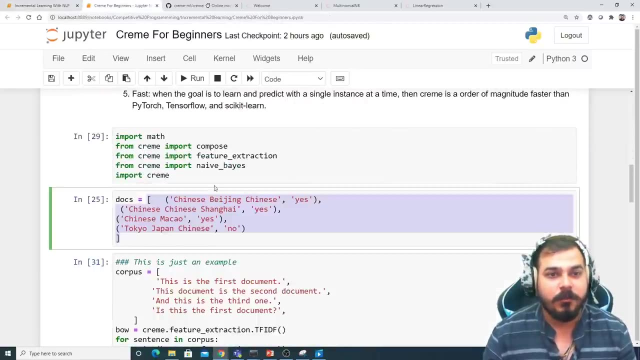 so you want to see different approach also. so i have written tf, idf. then the second function is basically multinomial. nape bias with alpha is equal to one. i hope this is pretty much simple. okay, compose is missing. where is compose library? okay, so let me just import the compose library from here. okay, 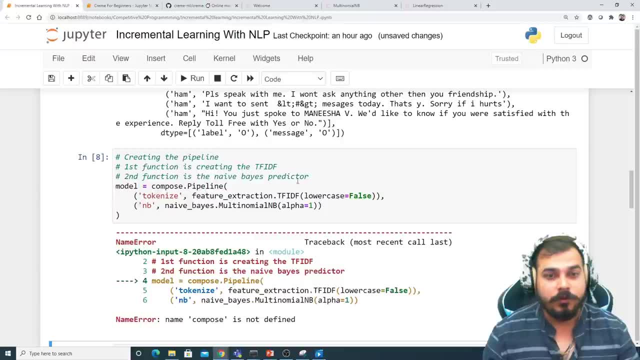 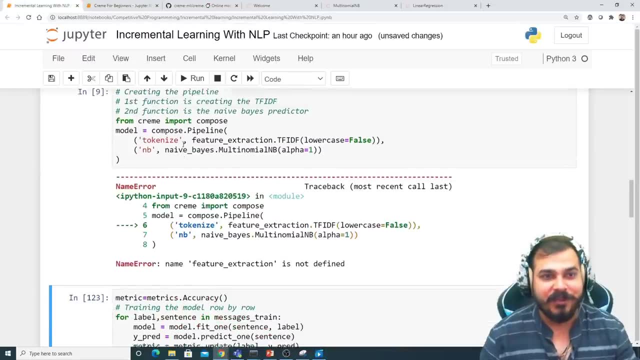 i hope so it works. i know this is the first one. this is the first one. there will be some more error because i have to use this feature, extraction everything. so i am just going to import everything over here. okay, just to, because this is another cell, right? so 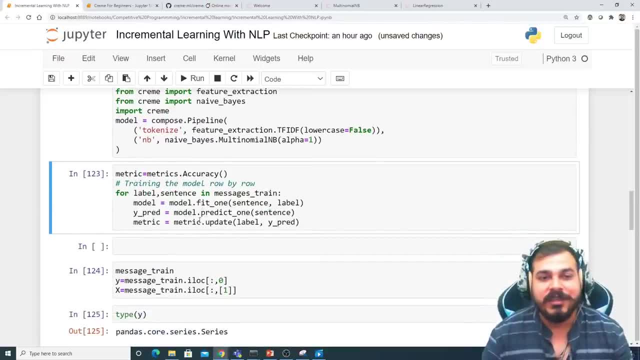 this is done right. our pipeline is actually created now. see when i am training, with my training data set also right, or any new data? we will also able be able to track the accuracy. we will also be able to track the accuracy always. remember that now. now in order to 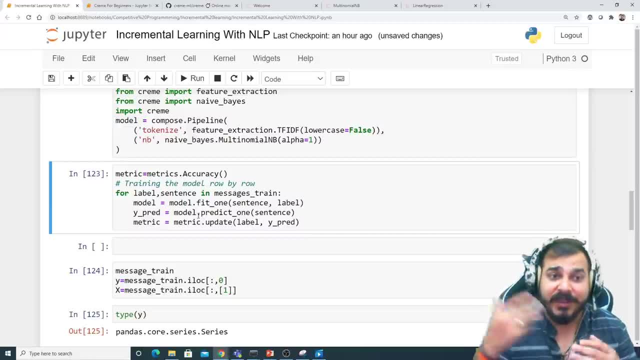 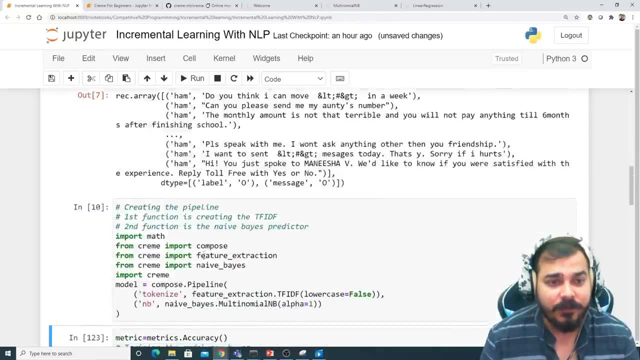 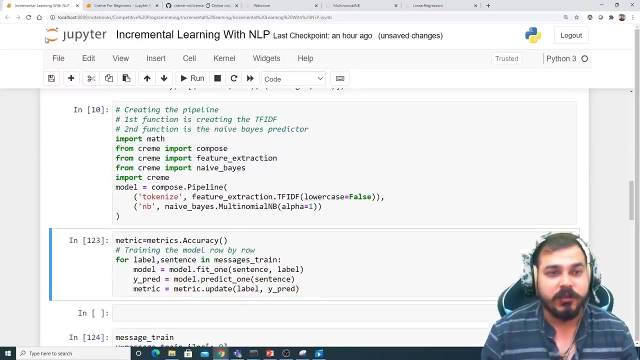 in order to basically track the accuracy. we will also be able to track the accuracy. what we have to do? you know that we have imported a library which is called as matrix. i guess somewhere we may have, uh, cremae, matrix, matrix, matrix, matrix. okay, so what you can do is that you 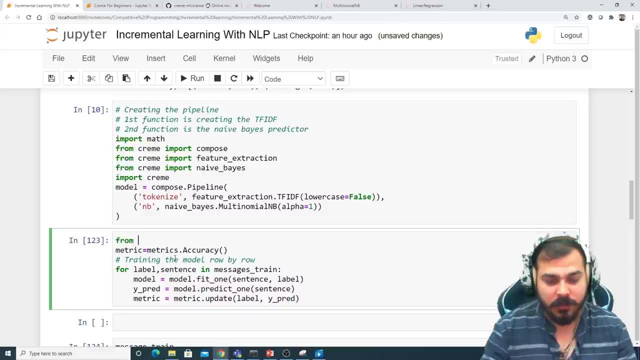 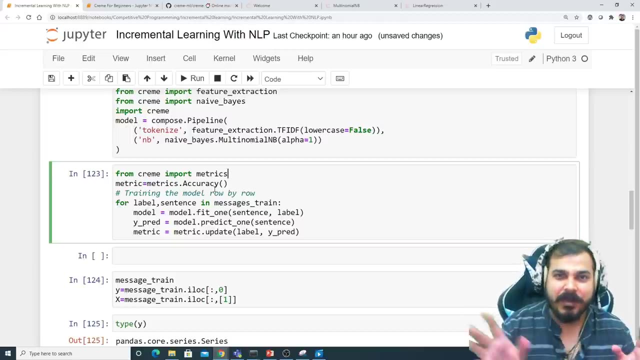 can upload one more library. you can say right from cremae import matrix: okay, so this matrix will be having metric metrics like msc mean squared error for classification problem. it will do that be having like accuracy and many more things. okay, you can actually see. see, over here you can write. 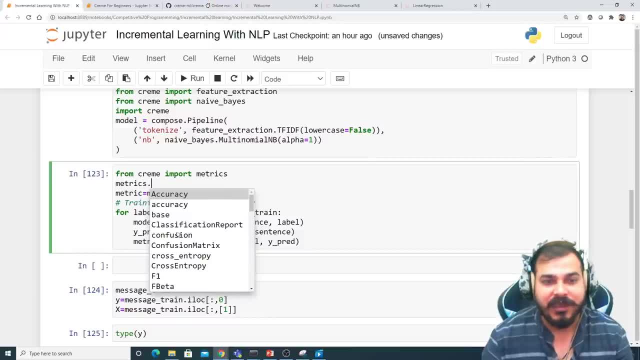 metrics dot tab. here you have a lot of things like classification, report, confusion, matrix, cross, entropy, f1, f1 also you have. so any kind of metrics you can basically use again, it has a lot of metrics, guys. so. so this crema library is becoming very much popular. so here what i've done is that i've 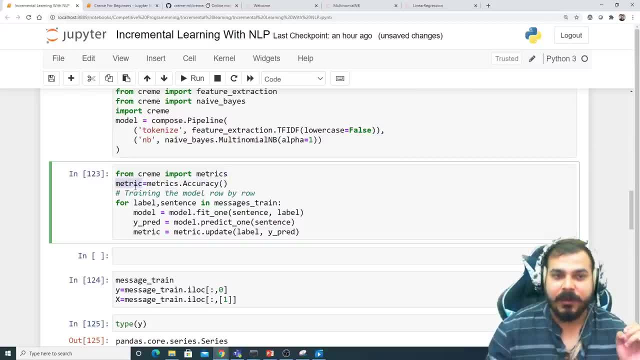 taken metrics. i've used the accuracy inside this metric parameter. now, this metric, you know when we will be updating. this will basically be getting updated with the newest accuracy. now, one thing that you need to know is that, as my model is training one by one record and that accuracy 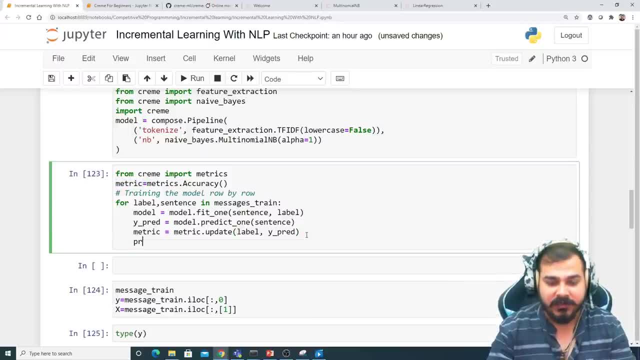 will also get accumulated. so if i, if i write something like this: see what is happening over here, right guys, and please make sure you see the video guys for label or sentence in message underscore: train now i'm training with all the message underscore: train all these particular. 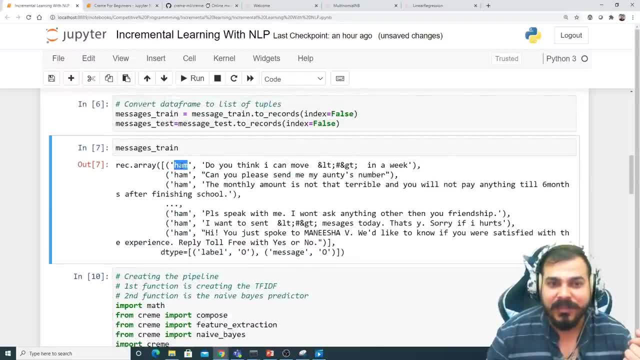 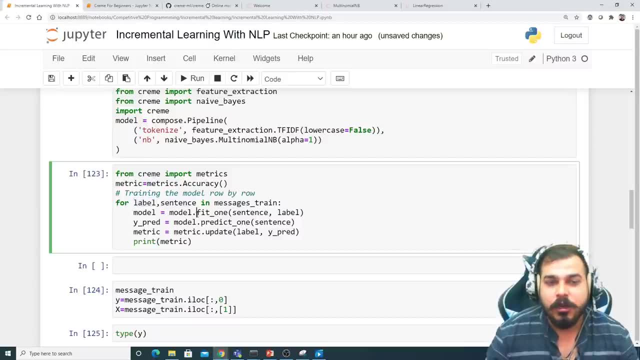 values. you can see that first is basically label. right, i will be considering this as my label and this as my sentence. so that is why i have used label comma sentence. then i'm writing model dot fit one with sentence comma label. okay, sentence comma label. i hope it is pretty much simple. 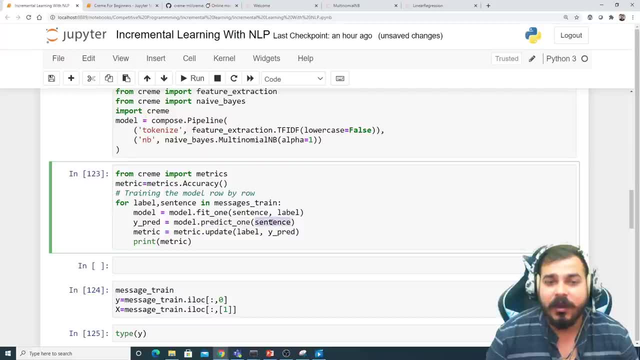 then i'm also doing the prediction, or predict, underscore one on sentence, and i'm actually capturing the y pred value to just see that how the accuracy is being followed for the training data set. now, this y pred, what we do is that we will be using this metric dot update. we are going 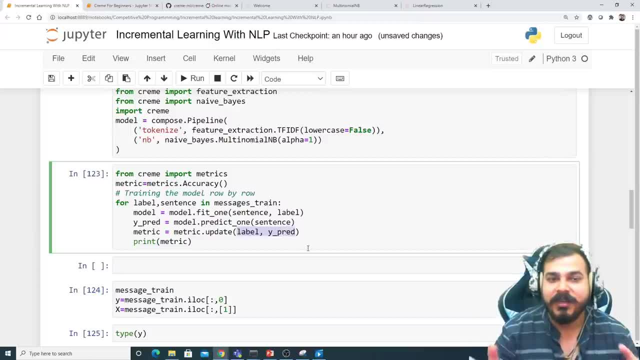 to basically compare label and y pred and what will be the difference? that will be updated in the metric. so, in short, this metric will be giving us the value of the accuracy and this will happen for every record, every record. it will be keep on updating the accuracy parameter. it will keep on. 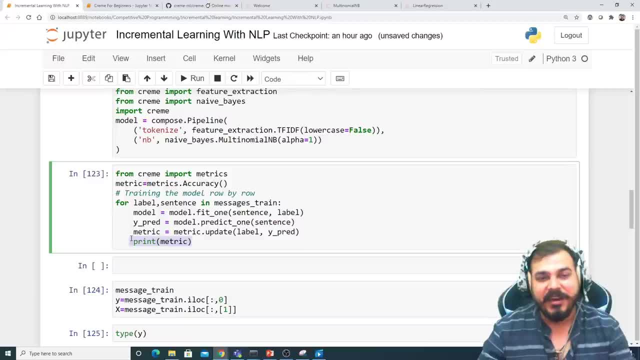 updating the accuracy parameter. i'll not print this metric for every iteration, guys, i'll just print it for the final iteration. so this is how you can see that how quickly this whole fit one has been done, because they are more than 5000 retard. now if i go and see my metric, you'll be able to see that. 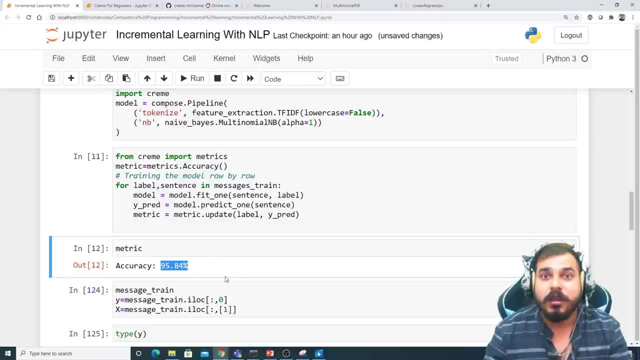 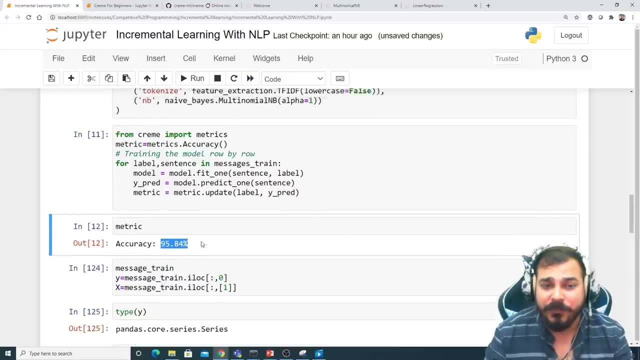 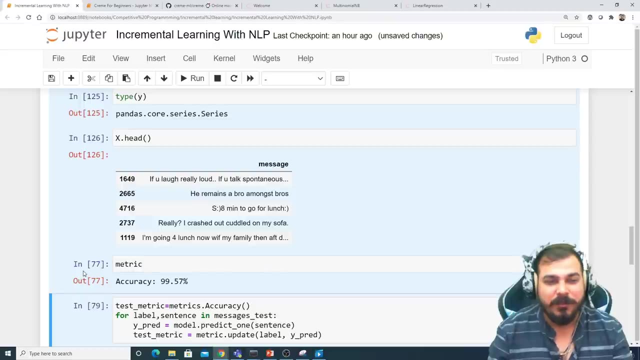 the accuracy that we are getting is somewhere around 95.84 percent for the training data. okay, for the training data, this, this is what we actually see over here. okay, uh, you can also convert this into x and y training data sets and all, but i'll not do it right now, or to just make. 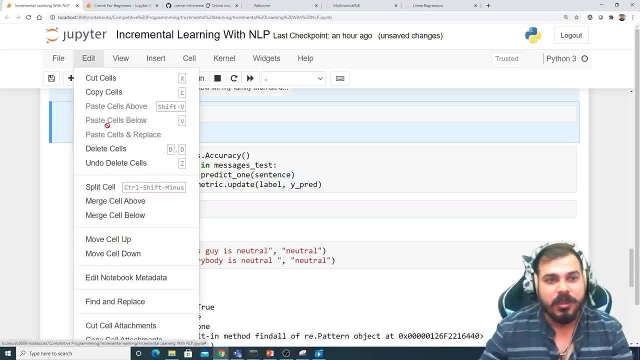 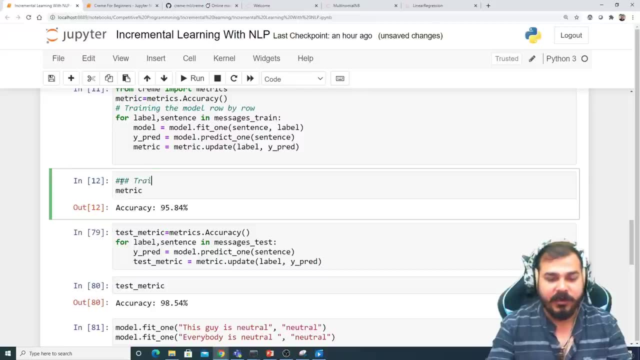 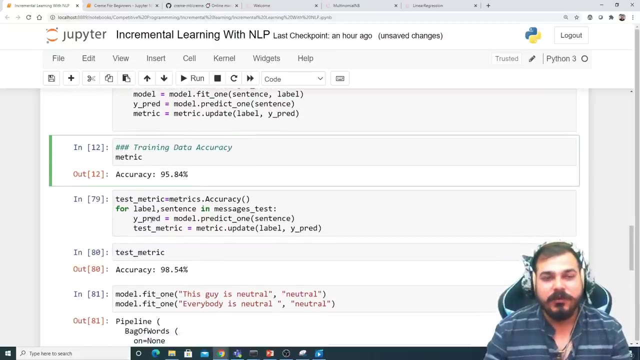 your simple uh things simple. so what i'll do is that i'll delete this. okay, now, this is basically with respect to my training data accuracy, so i'll just write it down over here: training data accuracy, but you can see, right, how fast it is, how good it is, right. then, after this, what we are going to do is that we are going to 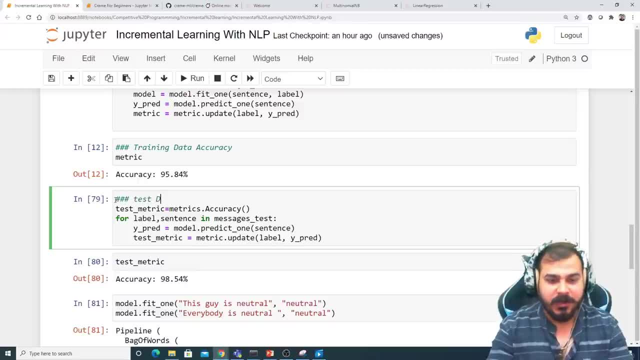 test it for test data accuracy. test data accuracy. now for the test data accuracy again, we are going to use metricsaccuracy, okay, and this. i have written it as test metrics now. this time i'll iterate through message underscore test. now i'll not do fit, i'll just do predict underscore one for. 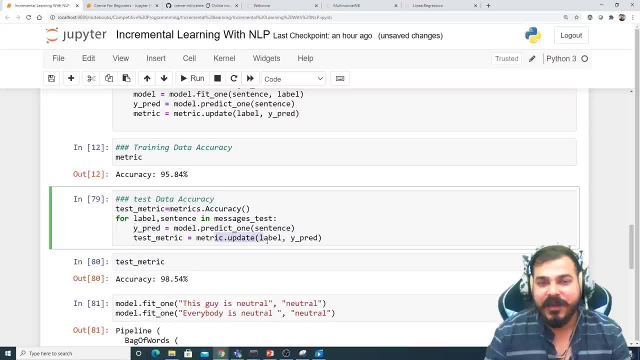 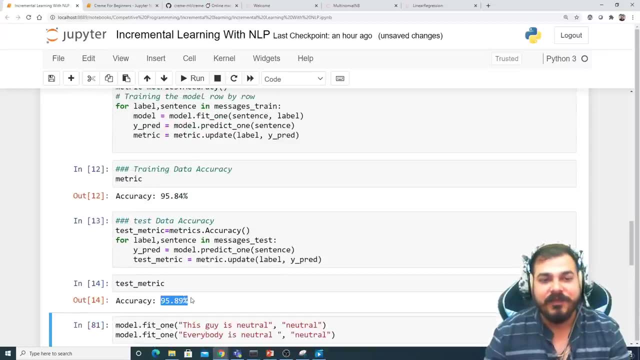 the sentence. i'll get my wipe read and i'll just update my metric parameter with label comma. wipe read. now, when we will be executing this, guys, you will be able to see that we are getting an accuracy of 95.81- 95.84 for the training data. right for the training accuracy and for the test accuracy. 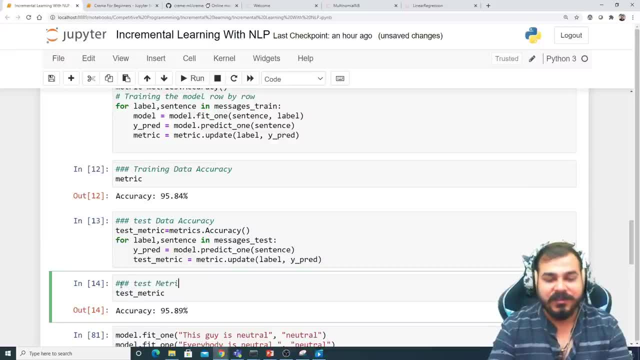 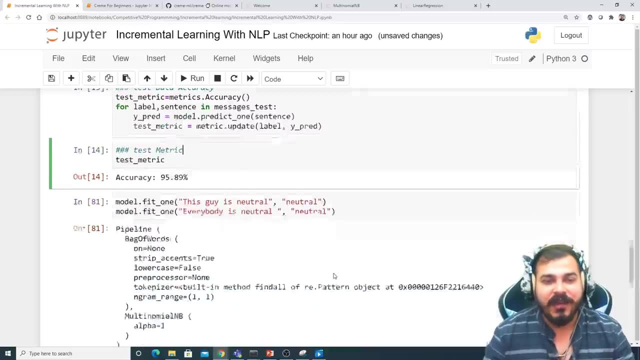 you will be able to see that there it is very, very less difference are there. so that basically means our model has trained properly. right it is. it has been amazing, it has been very good itself, and here you'll be able to see a lot of things itself right now. 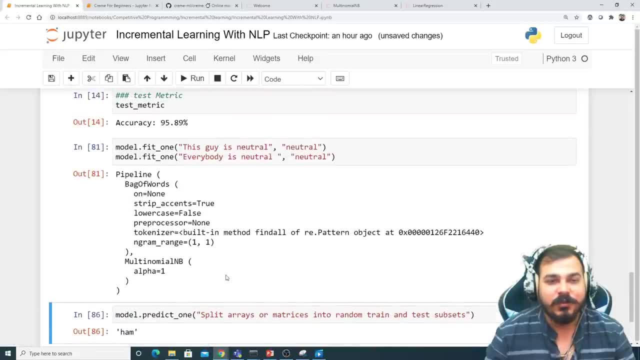 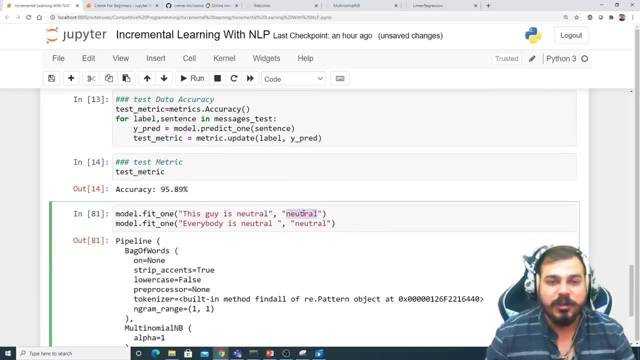 what we can also do is that we can uh, apart from this, you will be able to see that we can also train on new data set. right, suppose this is your new data set. suppose you want your new category. you can put it over here. suppose i'll say the guy is neutral, i can say it as okay. 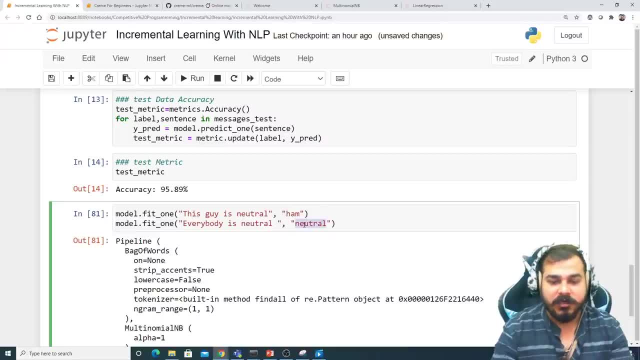 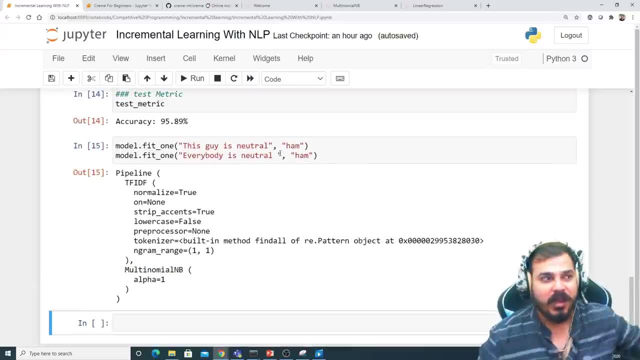 it is not a spam, it is a ham. uh, everybody is neutral. it is a ham, right? uh, you can fit any number of data like that any number of times. and this is where live stream data will come into picture, because live stream data- suppose you are getting one one, one data every time you are. 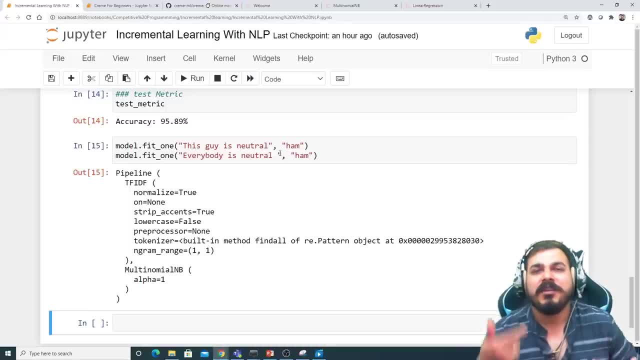 iterating through that and you keep on executing with fit one, fit underscore one and again. i have shown you from this particular example. you can also add any new number of categories, like: maybe you can add categories like neutral, spam, ham, neutral, anything, and here you can see that every. 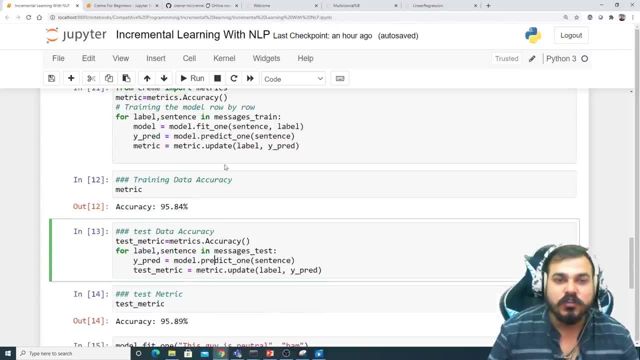 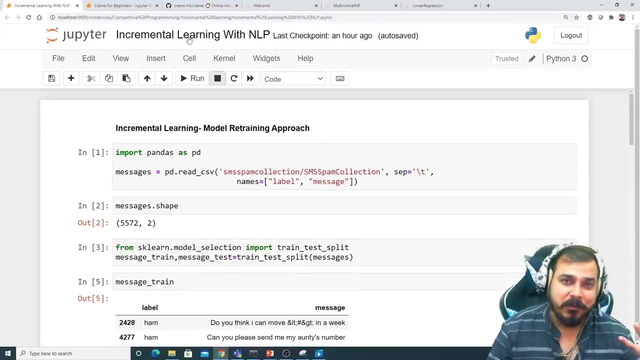 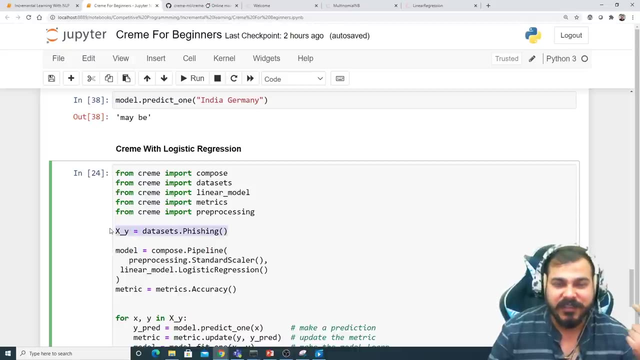 time, you'll also be able to monitor, as you are doing, fit underscore one with respect to each and every uh records. now, this is how incremental learning model retraining approach works, guys. if i take an example of one more like logic regression. so here you can see that i have taken a data set which is called as phishing data set. 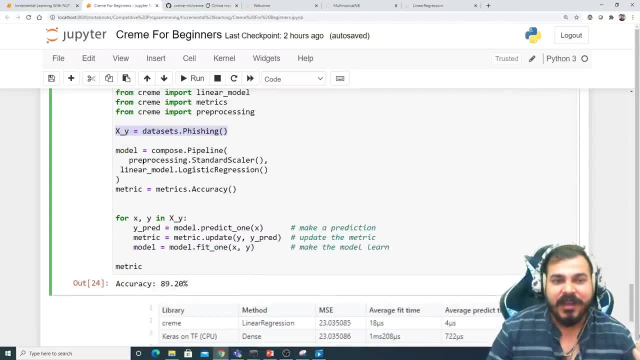 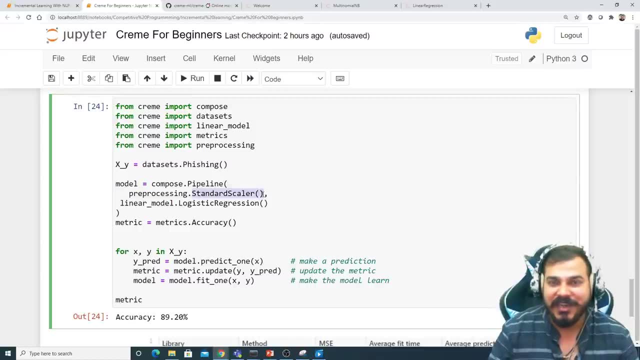 this is actually present inside the creme library itself. again, we have created a live pipeline and here now you can see that we have used pre-processing. inside this pre-processing, we have used first of all standard scalar technique. that is, basically we have done standard scaling and then we have applied logistic regression. again, this logistics regression is present. 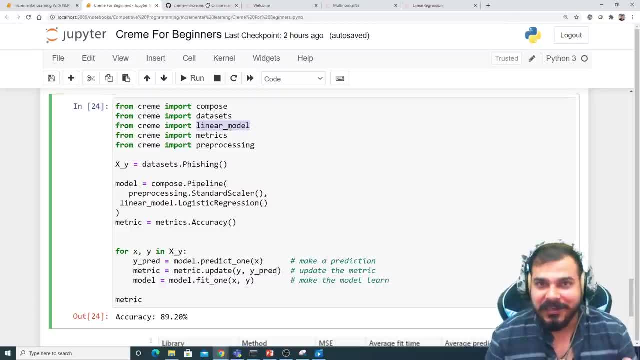 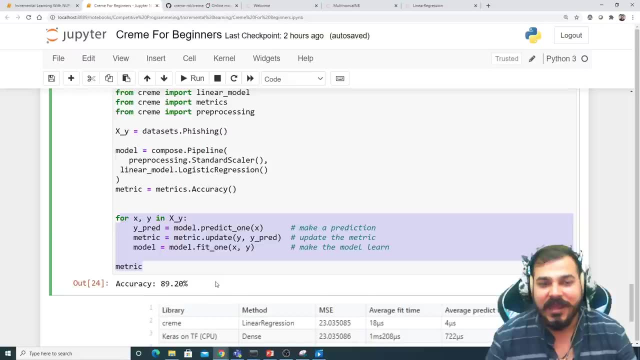 inside linear underscore model. in sk learn also, there is something called as linear underscore model, right, i hope you all know that. then again, uh, here also i am again taking matrix underscore accuracy and here you can see that i'm finding out, making a prediction, updating the metric and 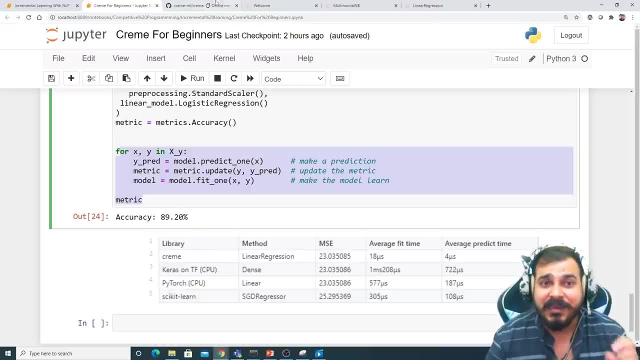 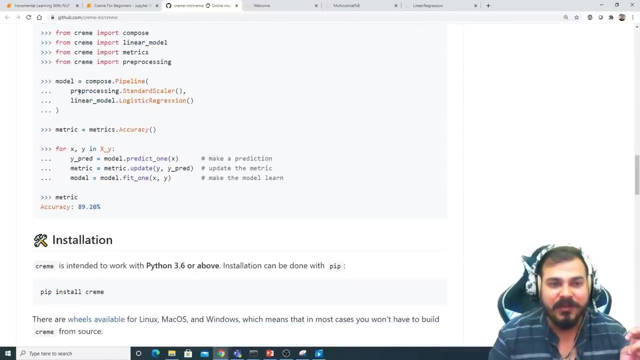 makes the modeler. so any machine learning algorithms. and again, guys, they are many machine learning algorithms. you just have to follow this github, you have to follow their documentation. i've taken this particular example from here itself and i have updated over there. so here i have shown you.